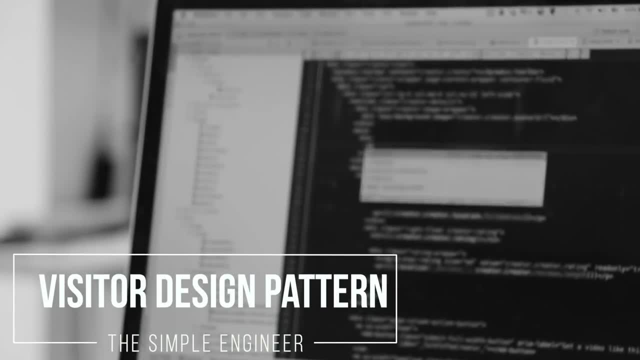 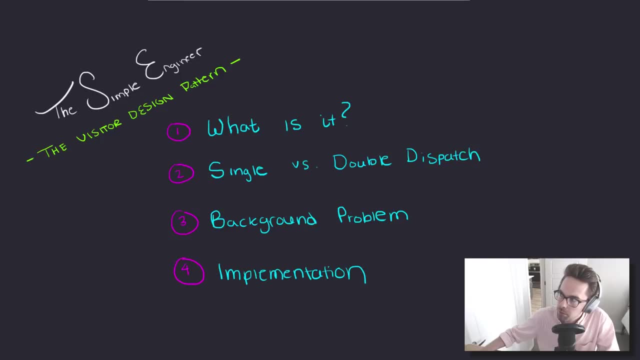 What's up, guys? Welcome to another video brought to you by The Simple Engineer. Today, we're going to be covering a cool topic known as the visitor design pattern, And the visitor design pattern is probably one of the most complex and underrated design patterns from. 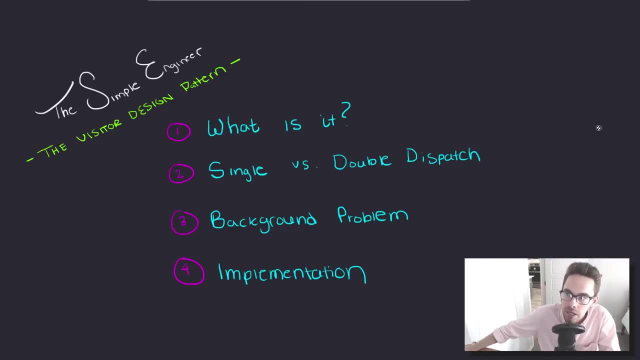 the original Gang of Four book, in my opinion. So in this video, what I'd like to uncover is first of all, talk about what exactly does this pattern solve, What's the issue that it solves, And then we'll dive into the theory as to why this pattern came to fruition. 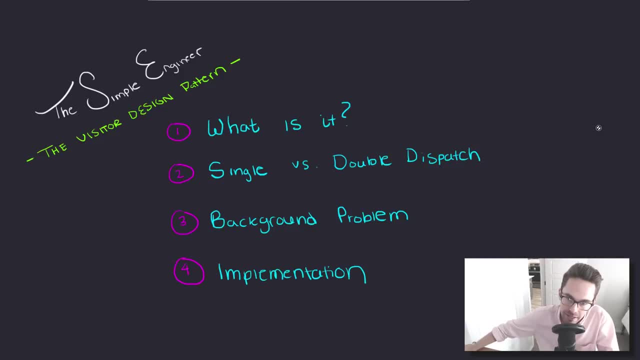 And that revolves around some object-oriented programming principles centered around polymorphism. And then number three: I've devised an example problem that will actually go over, and then we'll implement it using the visitor design pattern. So without further ado, let's just dive right into it. One of the things that I actually like is the description that 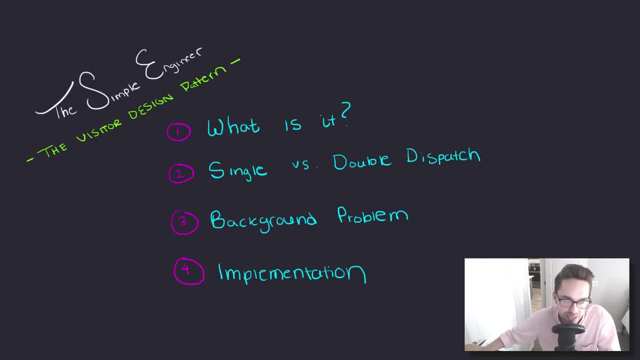 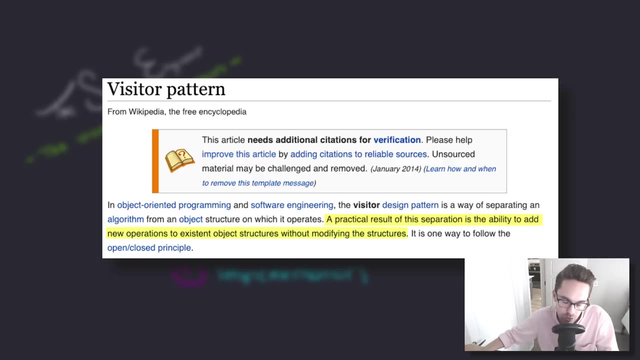 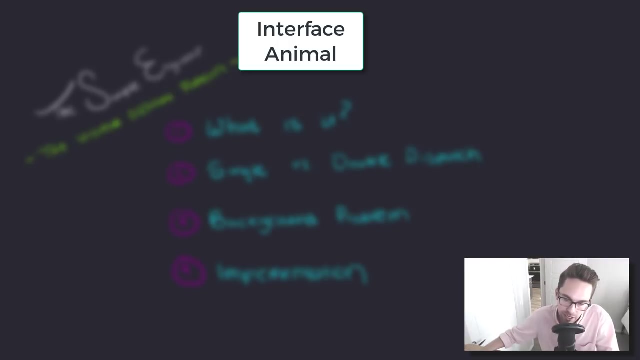 Wikipedia gives the visitor design pattern And what it says is: it allows us to separate new operations to existing object structures without having to modify those original object structures. So let's say that I have an object and it has a bunch of methods on it that are defined from some interface. So let's say I have an animal interface and I have 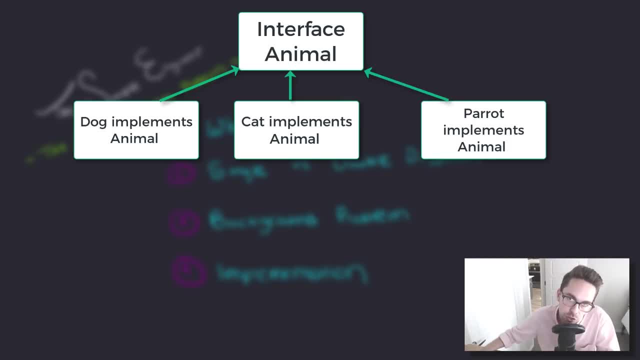 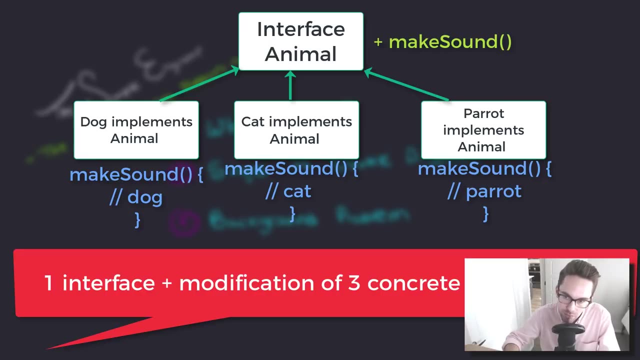 dog, cats, parrots, et cetera. Anytime that I add a new operation to one of those interfaces, to like the animal interface, I have to go and I have to update every single subtype to account for this new operation. So what I'm doing is I'm tightly coupling the operations that I'm 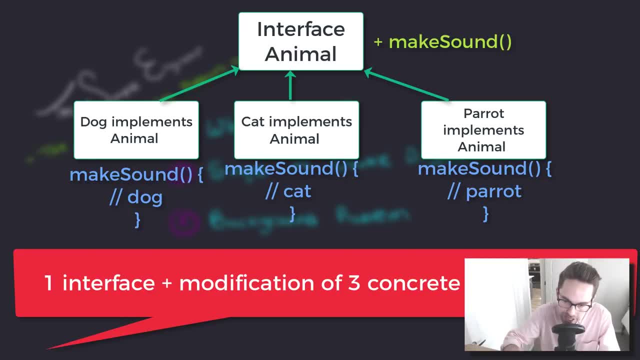 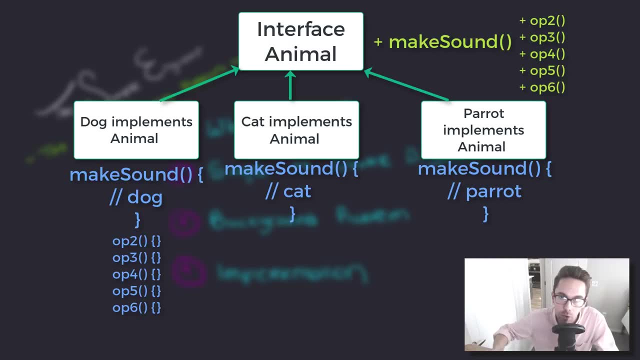 performing on these different animals to each individual animal object, And that becomes very, very difficult to maintain as we grow the number of operations on our classes. And in addition to that we are violating the open-closed principle, And the open-closed principle says we need to keep. 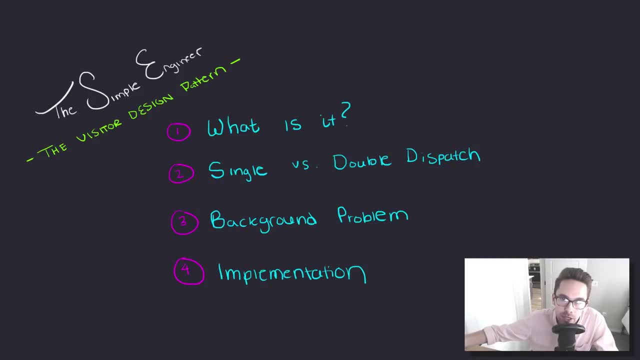 our objects. we need to keep our APIs open for extensibility but closed for modification. In other words, we don't want to have to modify the original API just to add new operations that interact with these objects. We should be able to do it in a very extensible way. So if I want to 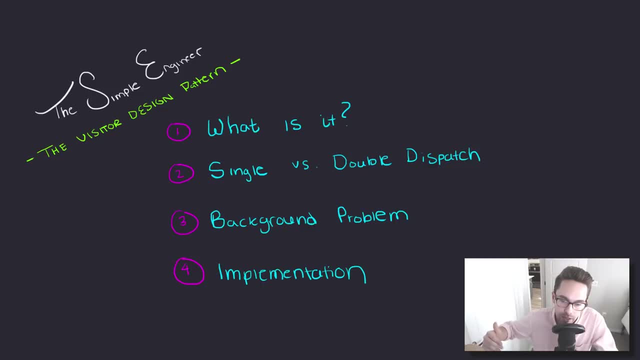 create an evaluator for an animal, or I want to create a new method that says: hey, give me the noise this animal makes. I don't want to have to modify the each individual animal class to be able to do that. So this is what the visitor design pattern solves. So to better understand what it. 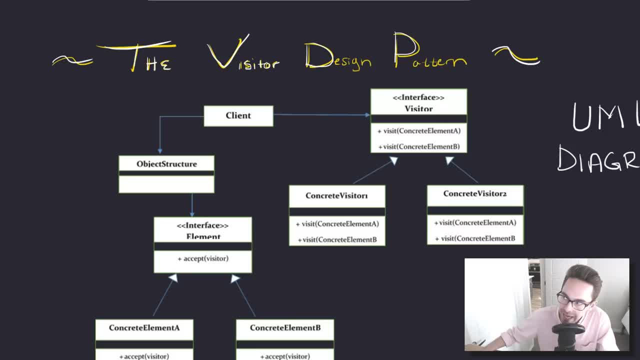 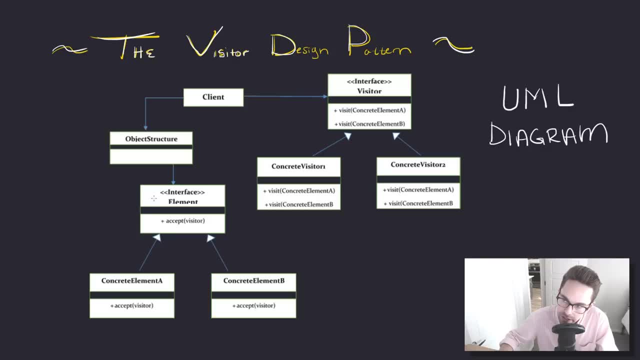 looks like from a hierarchical point of view. let's look at a UML diagram. So in the example that we gave, this would be essentially equivalent to the animal interface here. So let's say that this is an animal interface And concrete element A would be something like a dog And concrete element B would be something like a. 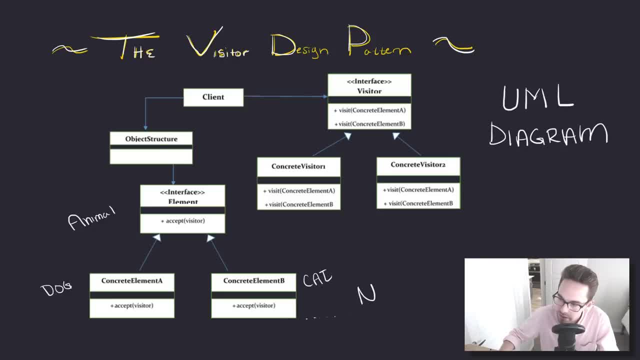 cat, And we could have N of these right. This could go on forever. And the simple change that we make is in the interface. so in the animal interface, which may already have a few methods, which is totally fine- We're just going to add one additional method, and it's: 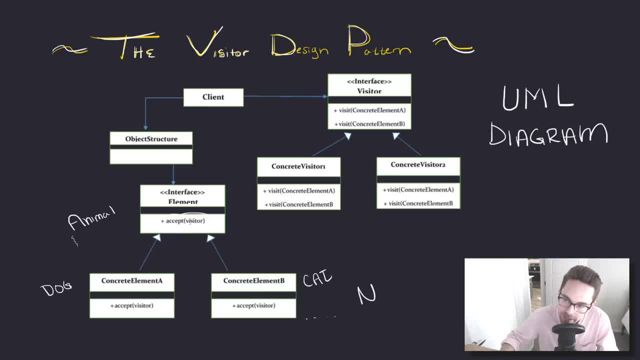 going to be called except And the except method is going to take in a visitor object And that's what we'll talk about in a second. So, as you can see how this modifies, the original concrete classes is just once. in the entire lifespan of these classes you have to modify once and it's. 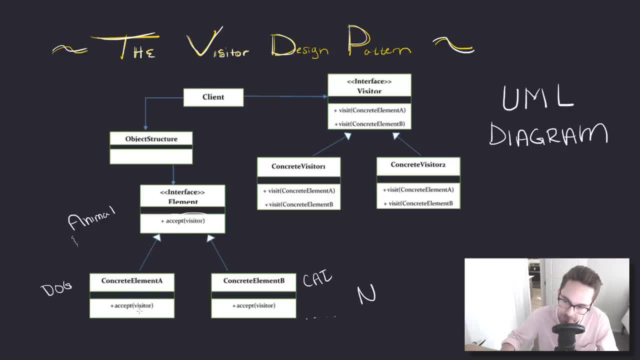 to actually implement. it's actually to add this, except method that takes in the visitor object And that's it. And this is going to be the extensibility point for all of our concrete classes, And we'll go into an actual implementation that elucidates this idea a little bit better. So this: 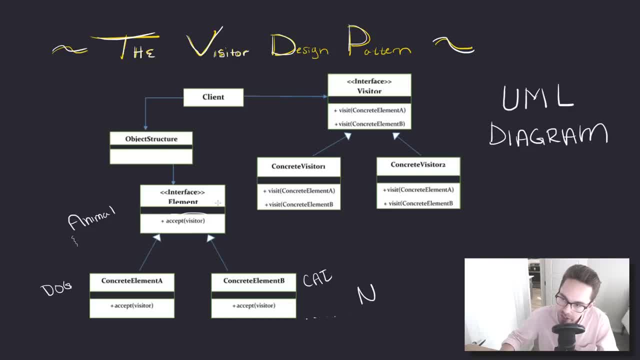 is the only thing that we basically change to our original data structure. we add one method to the interface and then we implement that method in the concrete classes. Now this is kind of the confusion point for a lot of people because, as you can see, we're essentially managing two pieces. 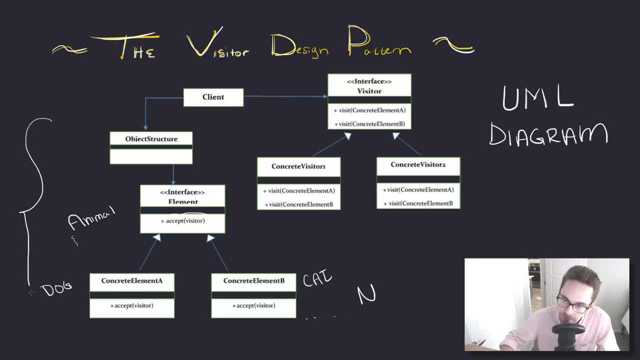 of hierarchy within this, this design pattern. This is the first piece of hierarchy, which is essentially all of our original data structures that we're dealing with, And the second piece of the hierarchy is the visitor data structures, And the way that I like to think about this is these concrete visitors are the 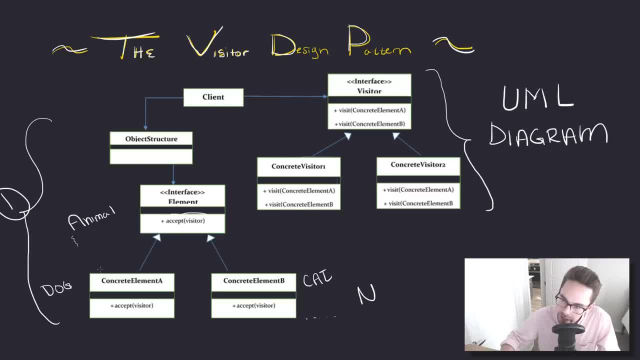 extensible operations that we perform on each of these concrete elements. So, in other words, if I want to add a method to all my animals, that's say, make sound or make noise, I can do that in these concrete visitors. I can make a make sound visitor And essentially what it'll do is it'll 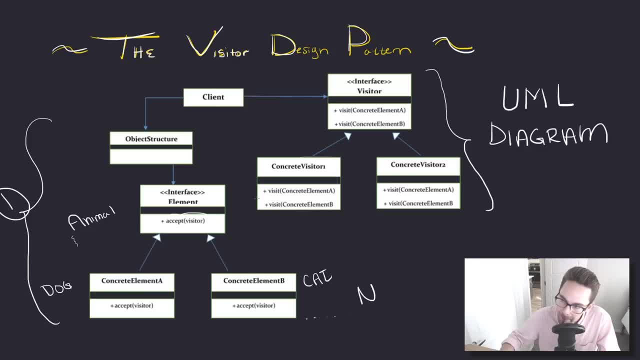 take in one of these concrete elements And when I pass it in it'll make the noise of this element, for example, it will bark, And if I pass in a cat, it will meow, And that's only specific to this entire visitor. So each visitor that derives from the visitor interface is going to be: 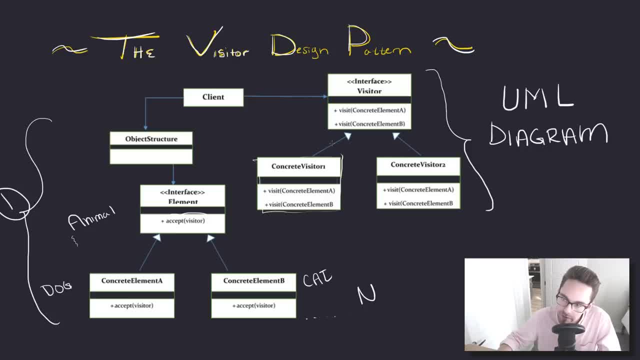 essentially a new operation or a new method that would have otherwise been tightly coupled to the concrete element itself, And that is the abstraction that we get using the visitor design pattern. So, for example, this could be a make sound visitor and this could 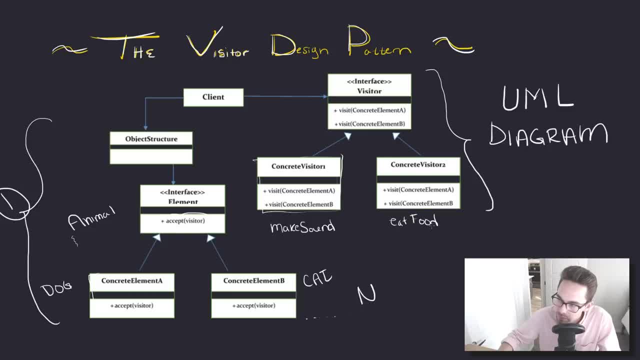 be an eat food visitor. And what happens is when we call this accept method in each concrete element, what we're doing is we're passing itself, we're passing in a visitor and we're saying visitor dot visit and we pass in an instance of ourself. So when we instantiate 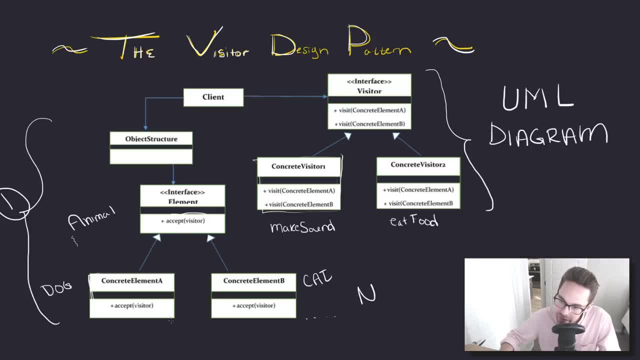 one of these visitors, for example the make sound visitor, and we pass it an instance of ourself, it will overload the correct method for make sound and our business logic will go into each of these visitors. So that's kind of just an overview of the UML for how something like this. 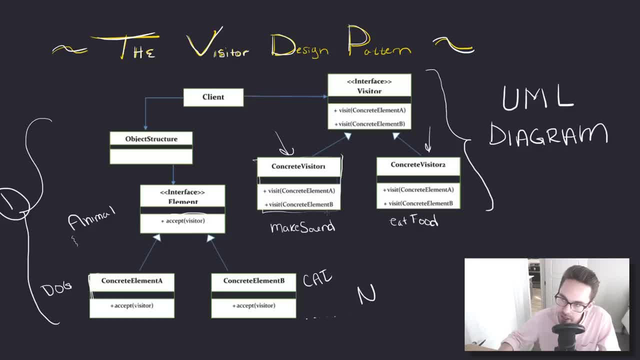 gets structured, But we'll look at this in more detail using a more canonical example that's a little bit easier to understand for something that's slightly more technical, But I did just want to get that diagram out of the way so we can understand the structure and the two pieces of hierarchy that we're dealing with in this. 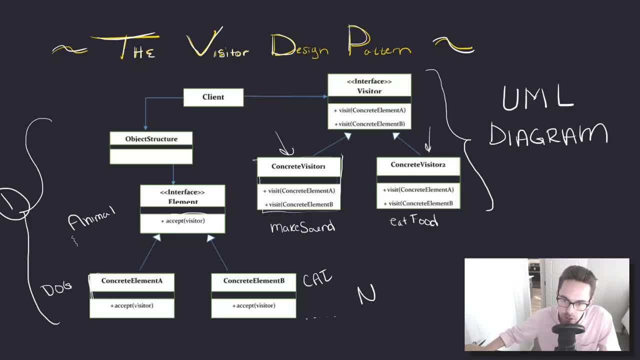 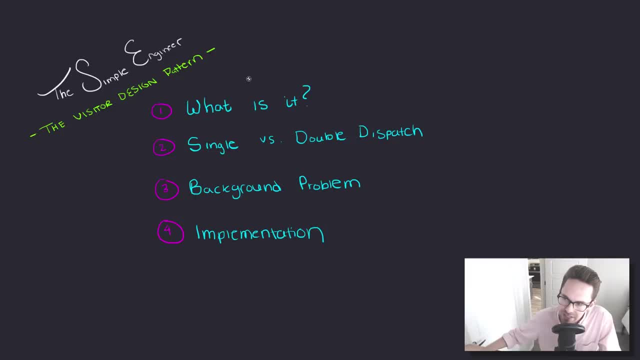 kind of polymorphic structure here. Okay, so, looking back, we we've covered the visitor design pattern, what it is, and the overall diagram, But let's talk about why something like this came to fruition, And it all centers around this idea of single versus double dispatch, And single versus double dispatch is 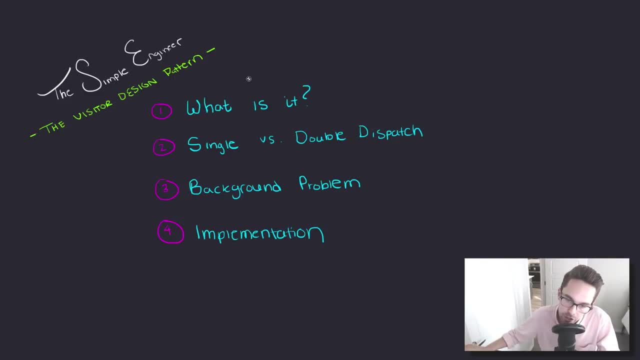 something that we're probably already familiar with, but maybe under a different term, And that term is polymorphism. In modern day object oriented programming languages like C++ and Java, they support single dispatch out of the box. It's something that comes with the benefit of 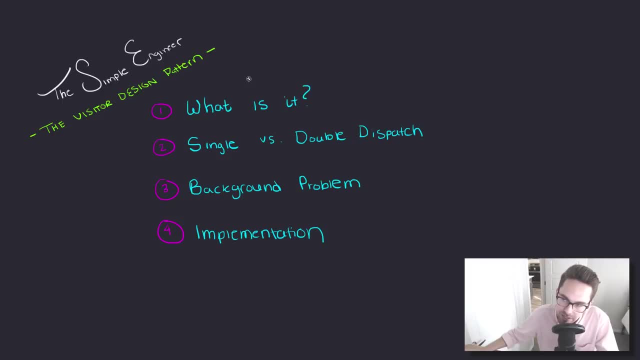 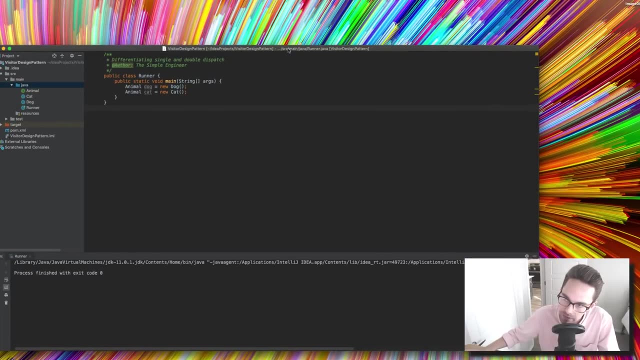 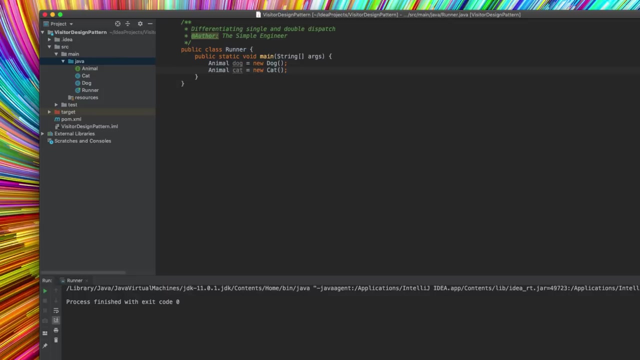 inheritance and polymorphism, But double dispatch is something that we're probably already familiar with, So let's go ahead and look at a use case as to what that is and where it fails. So before we explain the differences between single and double dispatch, let's first talk about what is single. 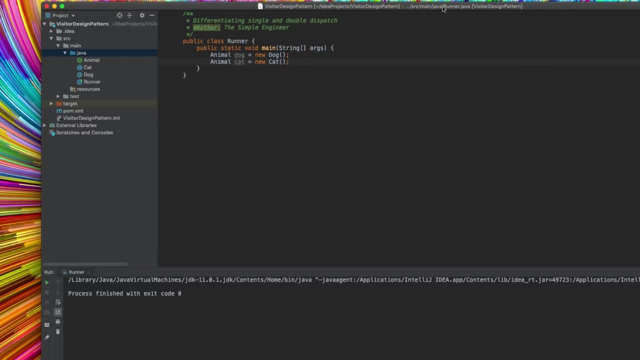 dispatch. I've gone ahead and I've made an example project here And just to quickly recap what this code is, I've created one interface And this interface is an animal And it has a single dispatch And it has one method on it called make sound. I've created two concrete implementations. 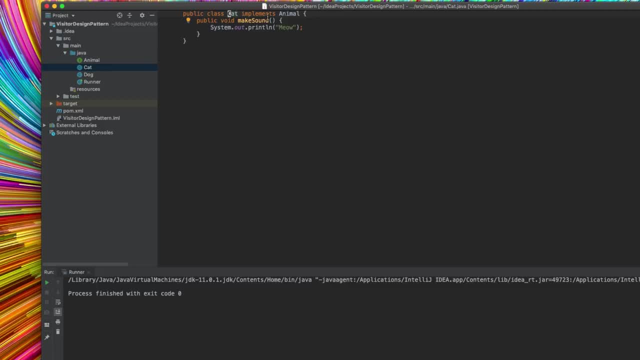 derived from this interface. I've called it a cat, which is a subtype of animal, And it meows, And I have created a dog, which is also a subtype of animal, and it barks. So what single dispatch allows us to do is we can declare or instantiate two different. 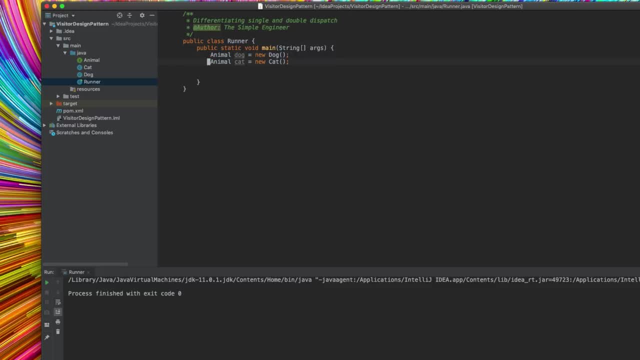 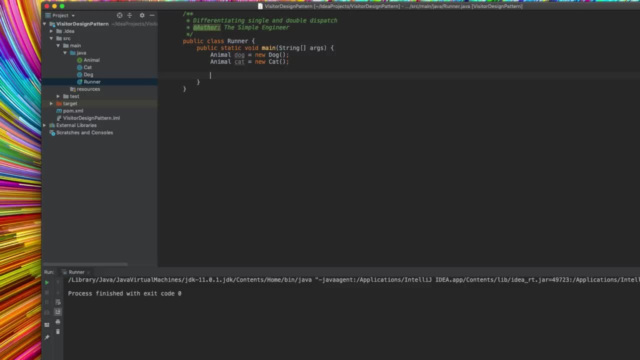 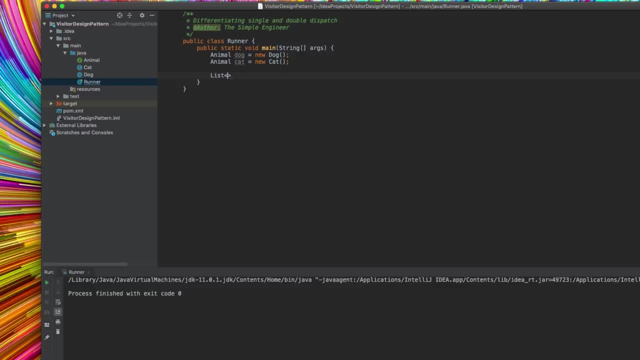 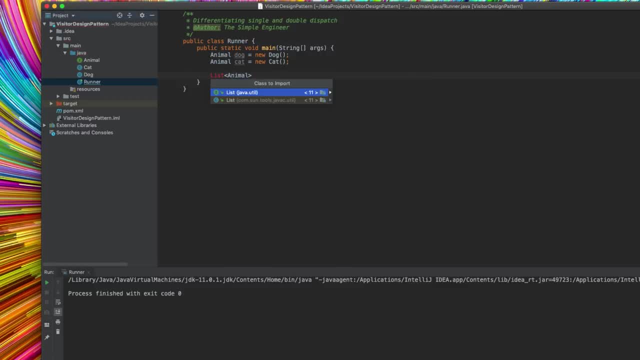 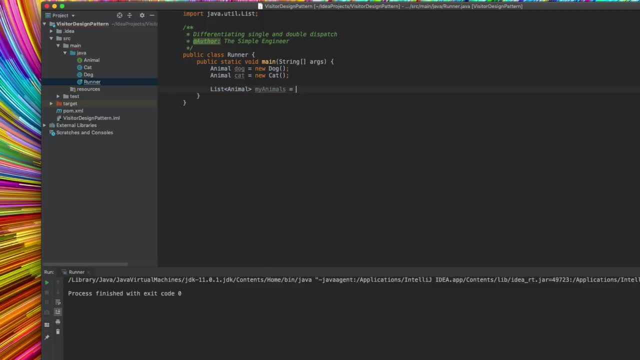 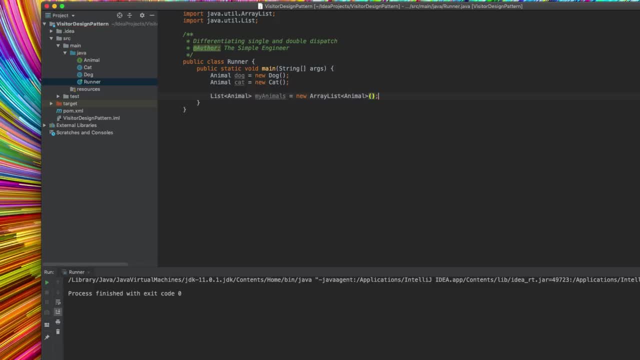 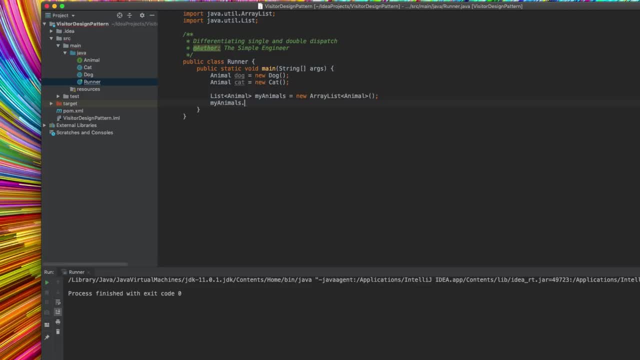 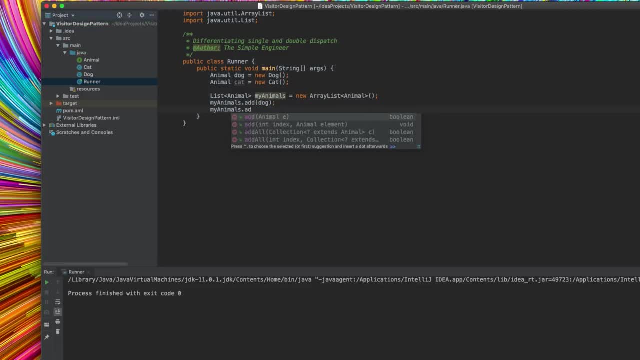 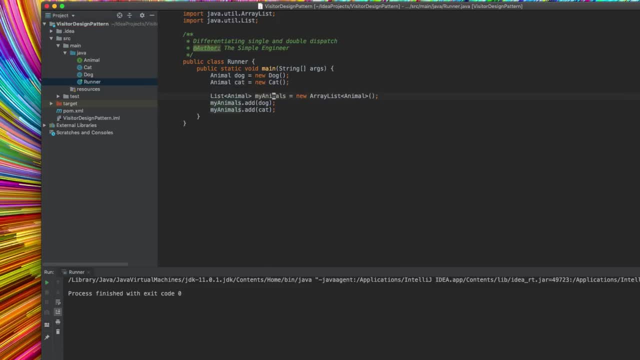 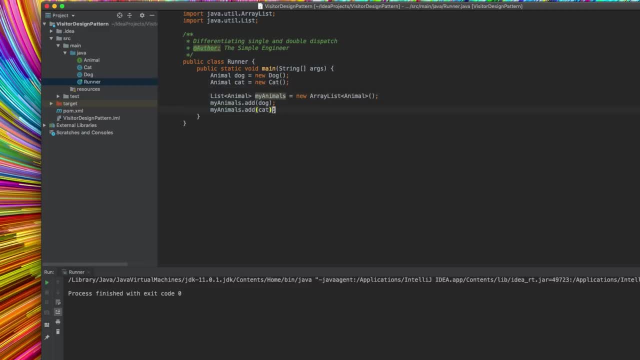 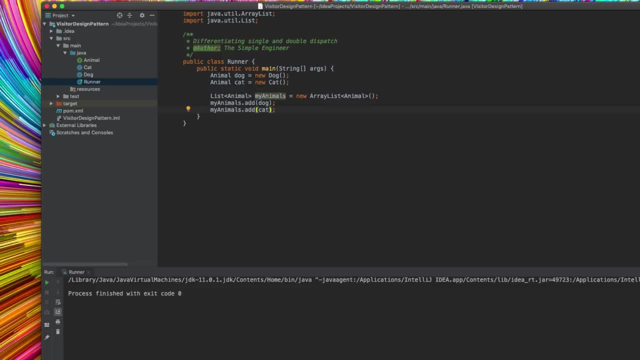 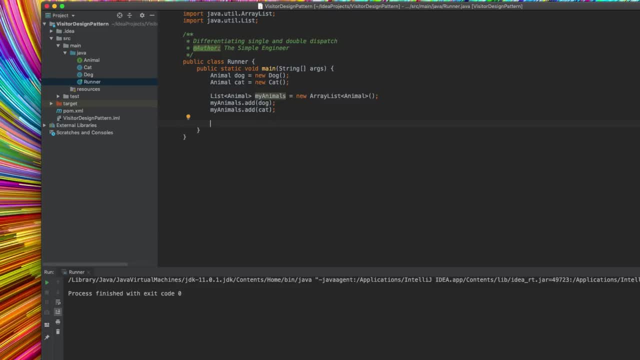 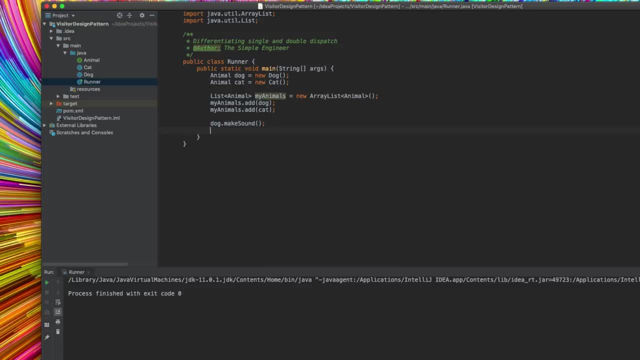 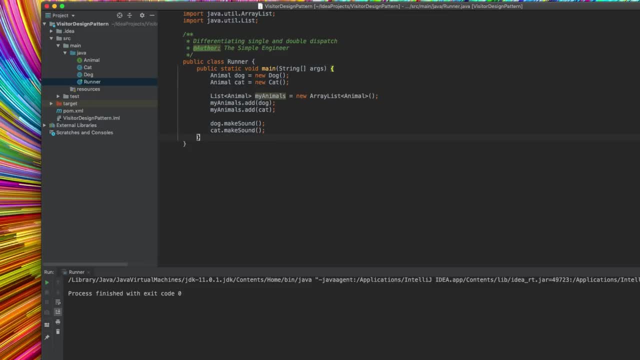 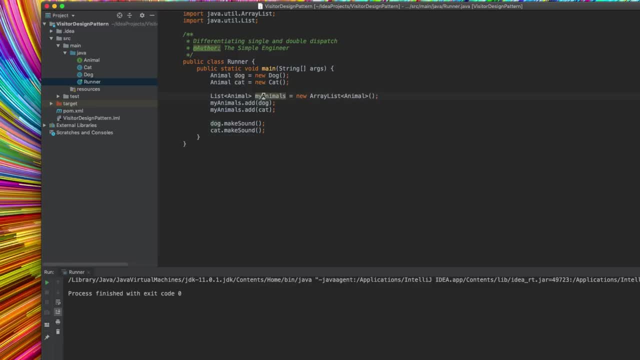 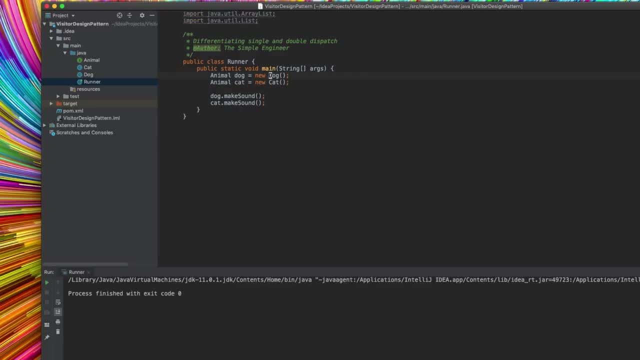 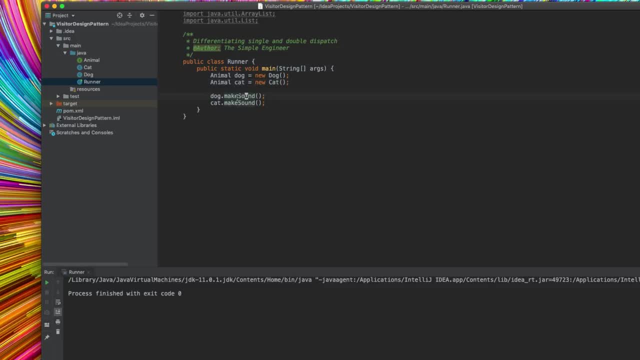 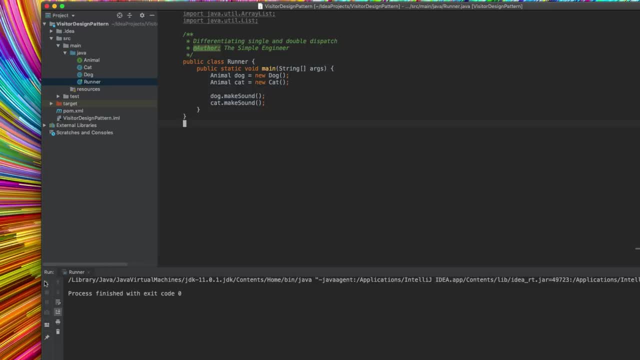 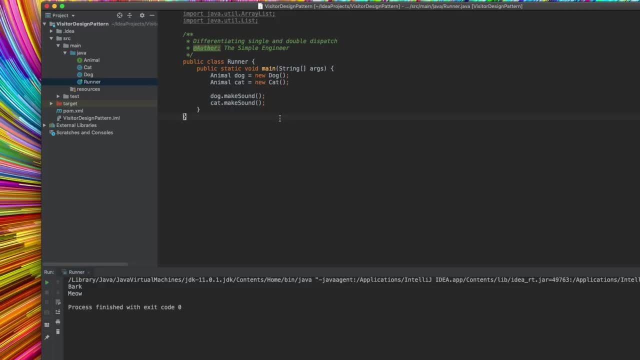 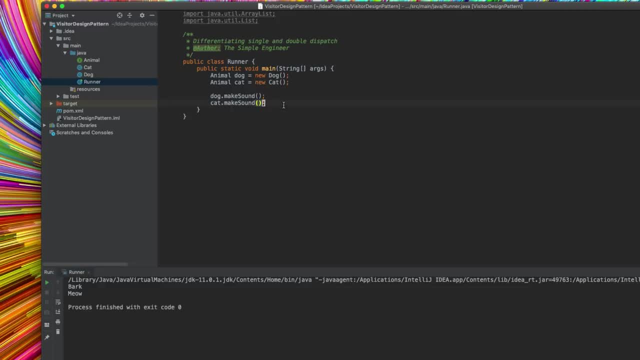 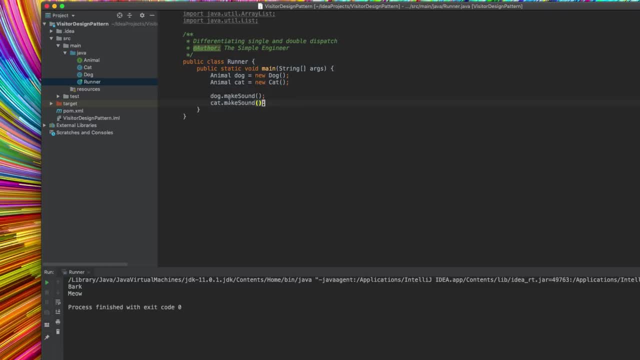 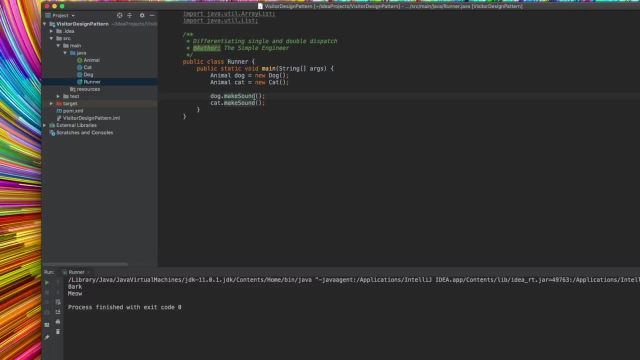 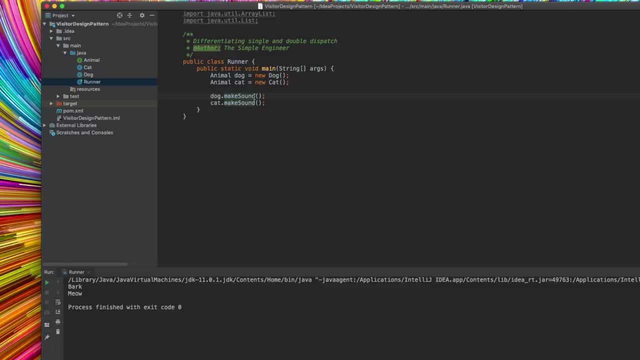 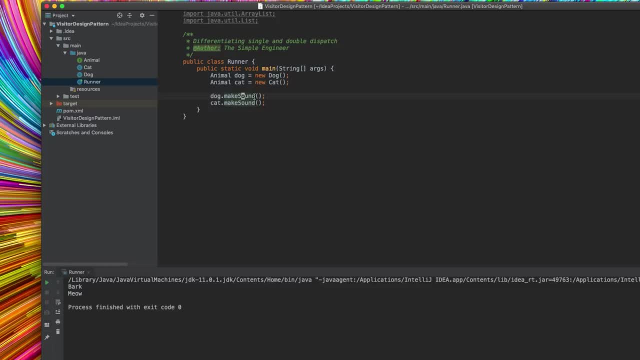 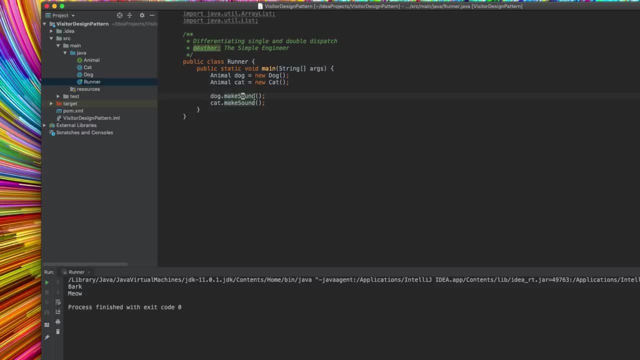 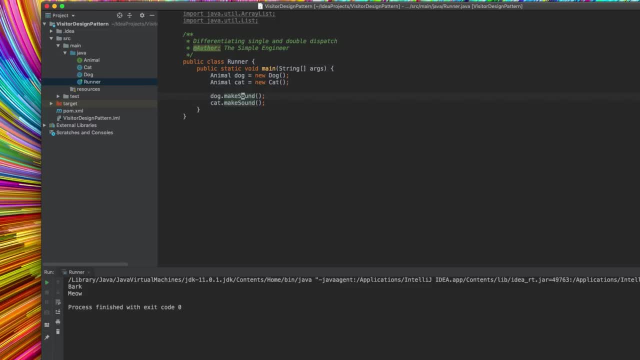 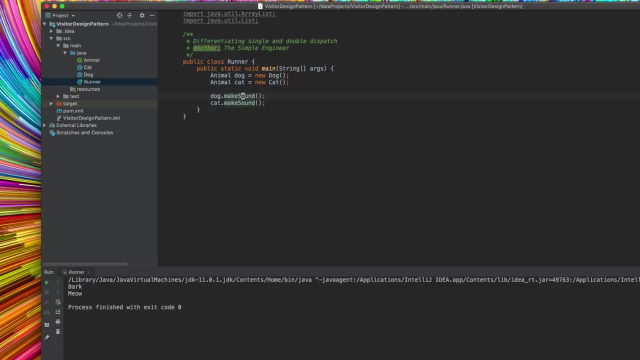 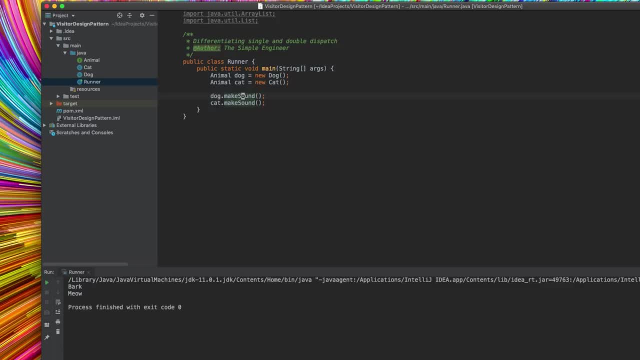 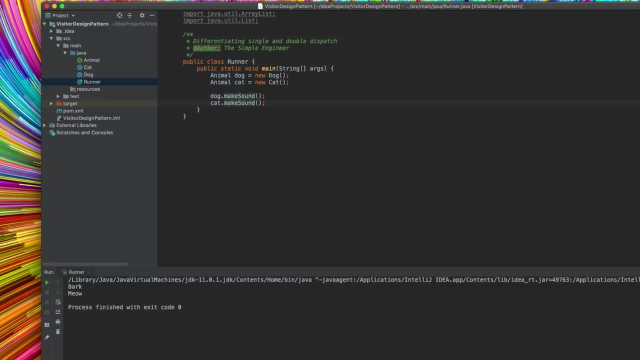 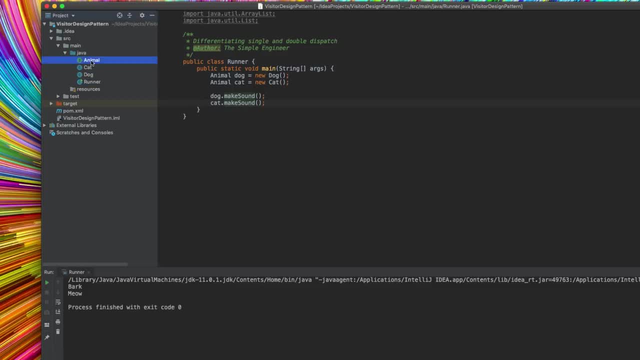 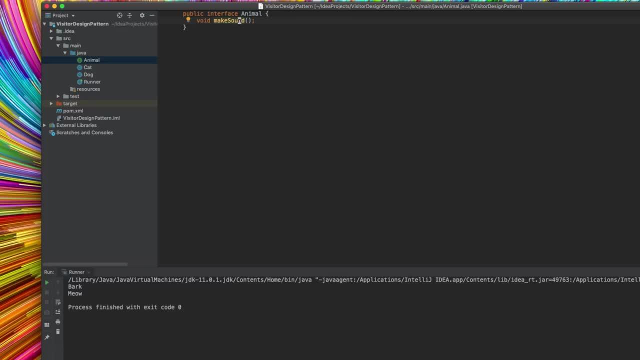 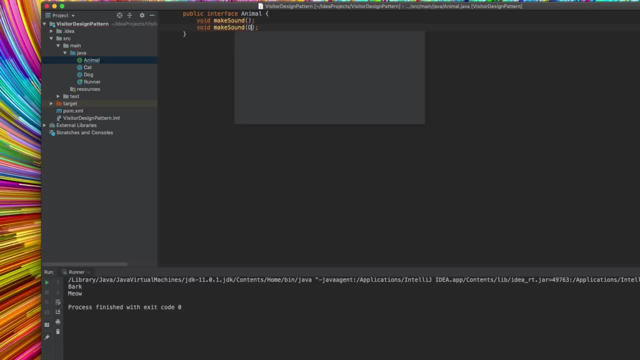 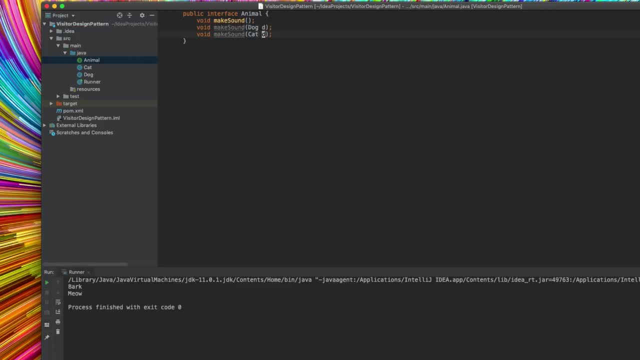 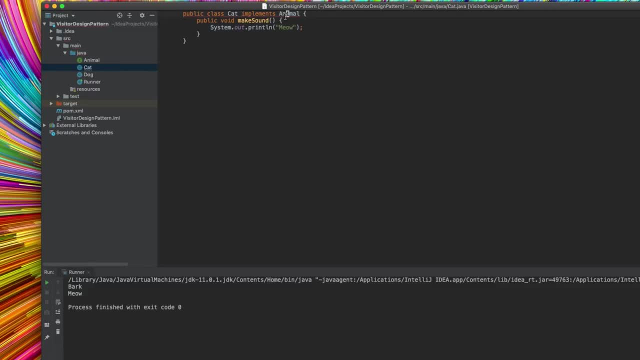 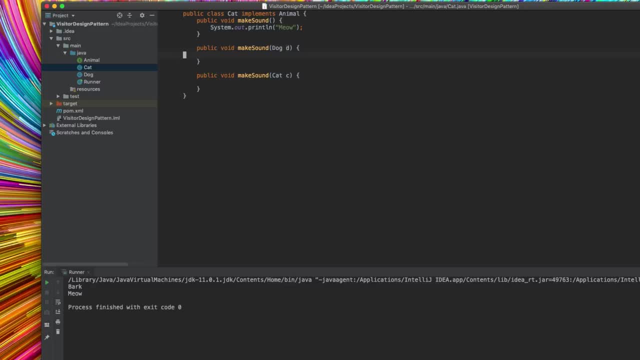 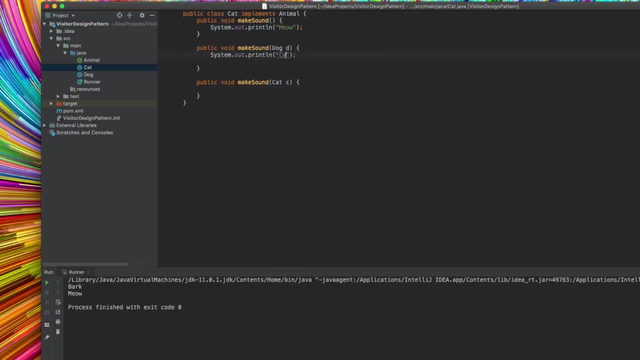 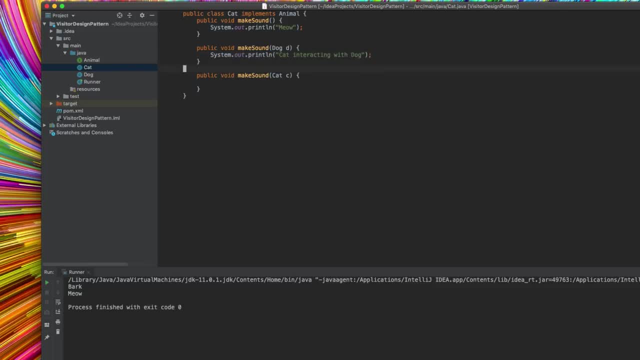 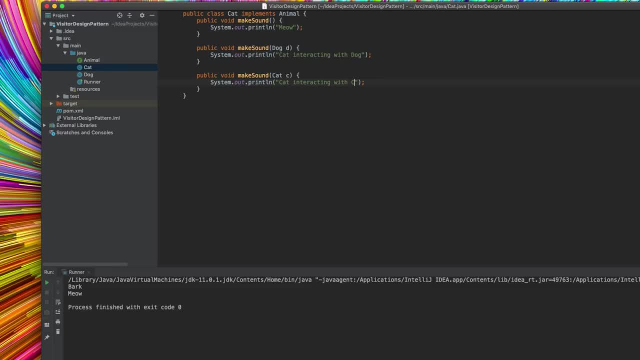 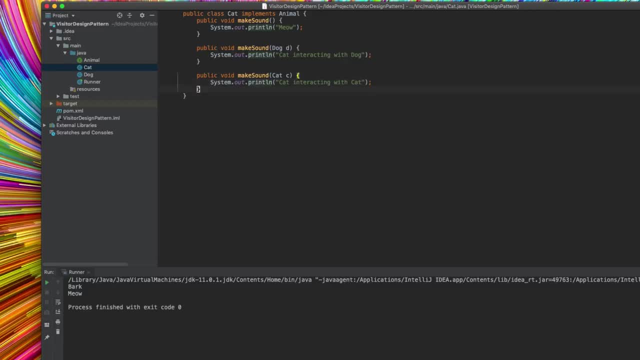 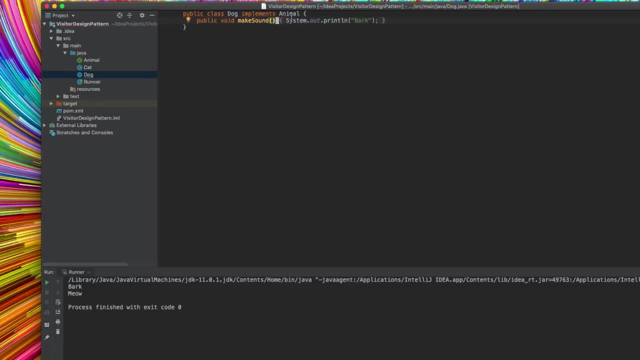 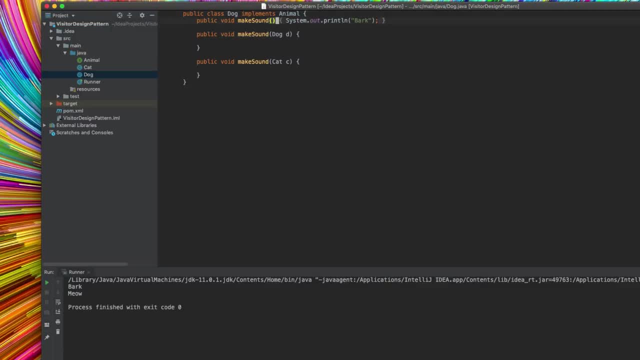 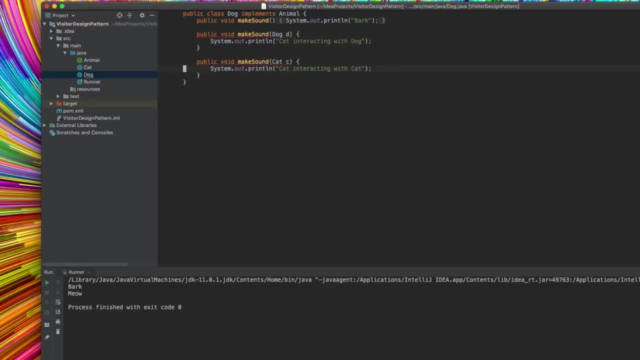 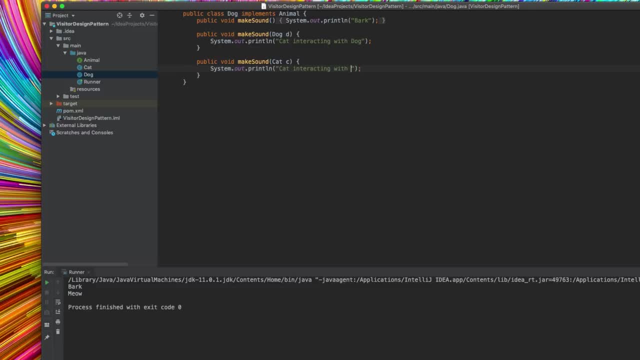 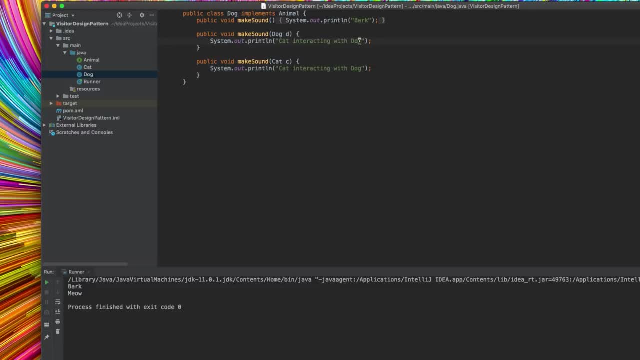 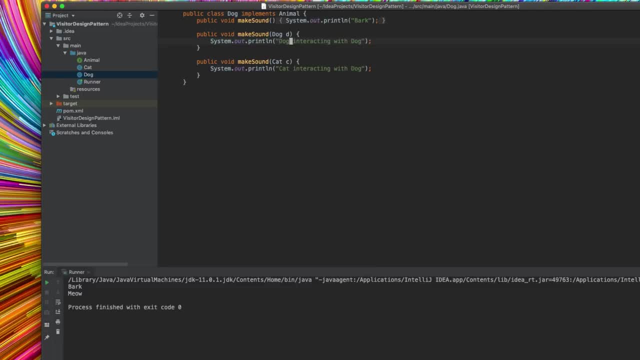 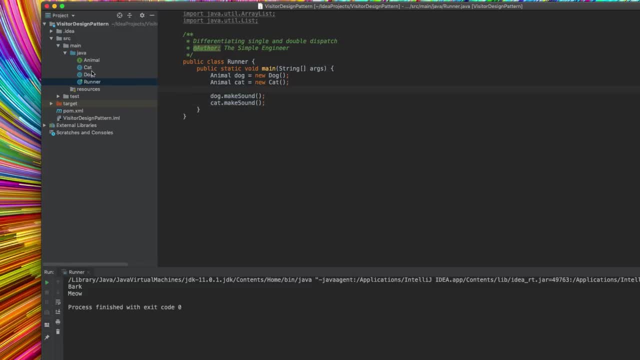 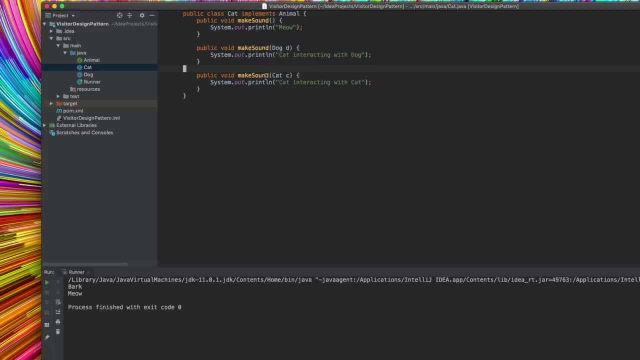 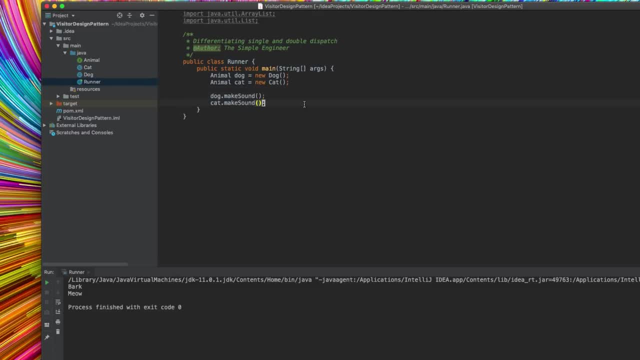 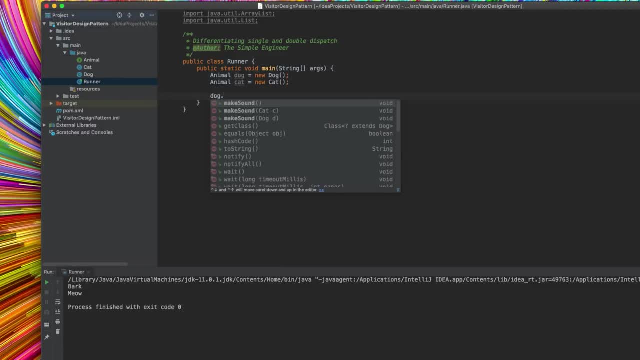 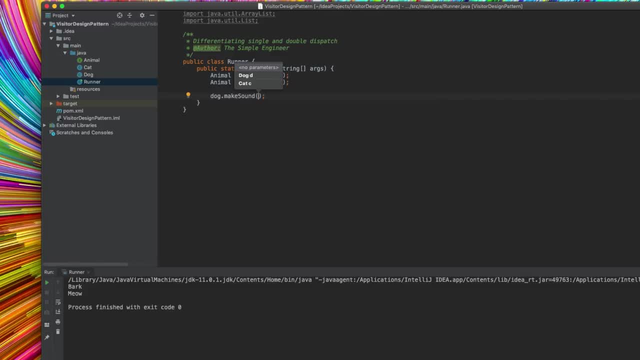 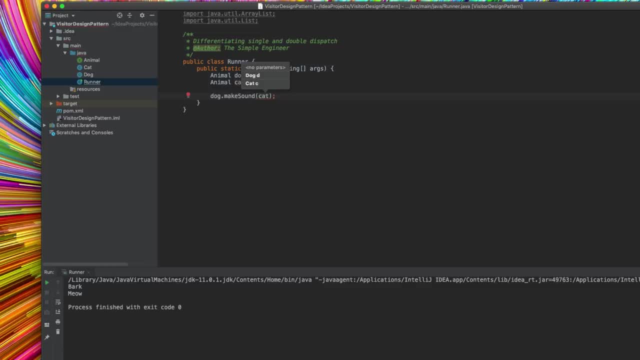 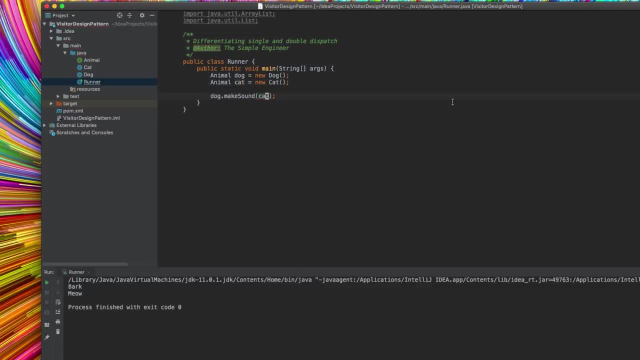 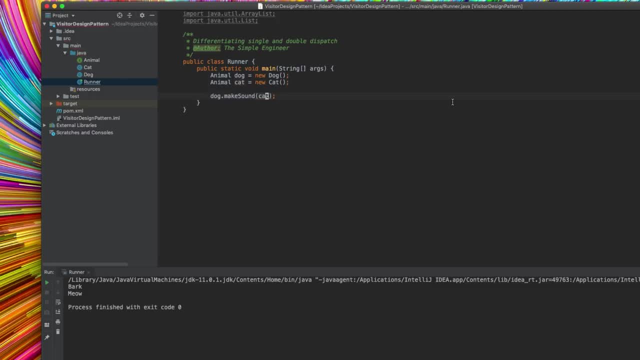 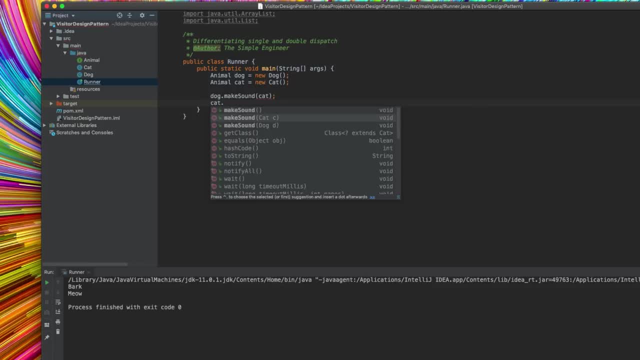 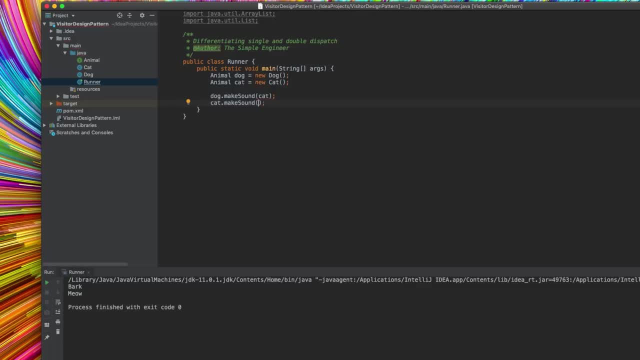 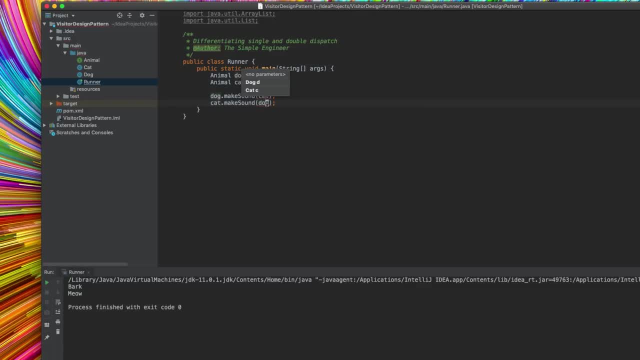 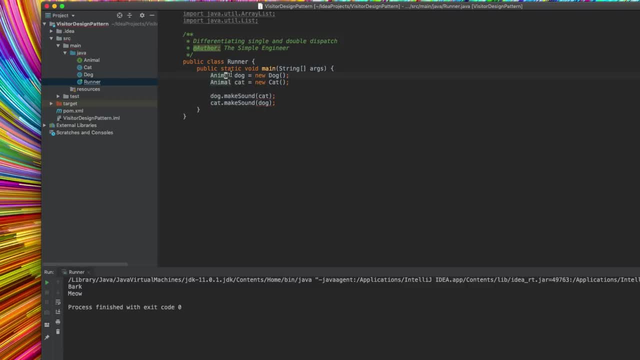 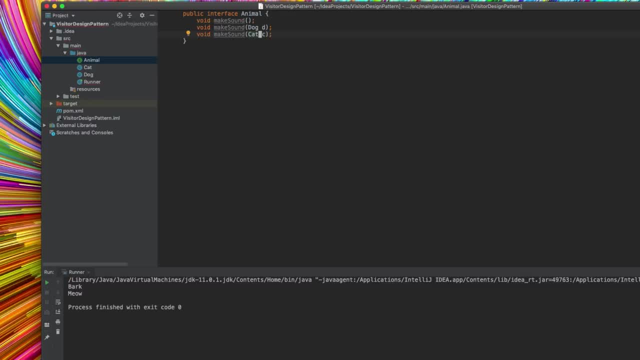 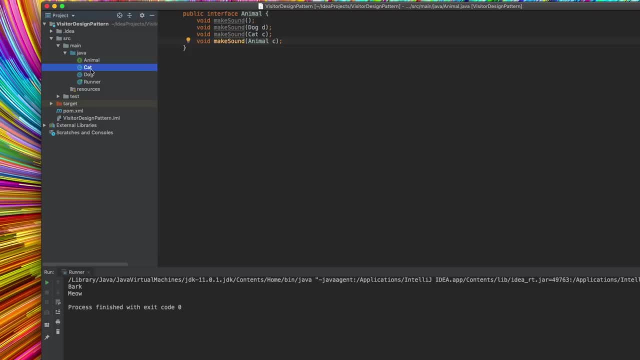 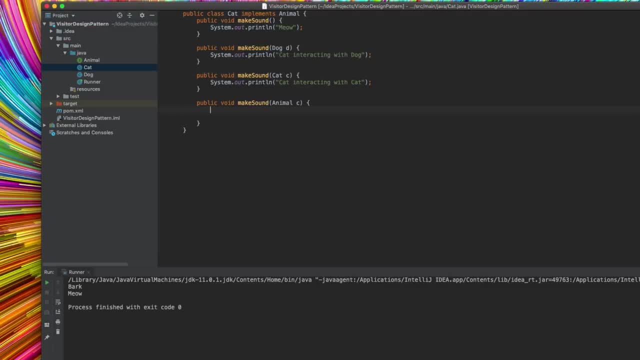 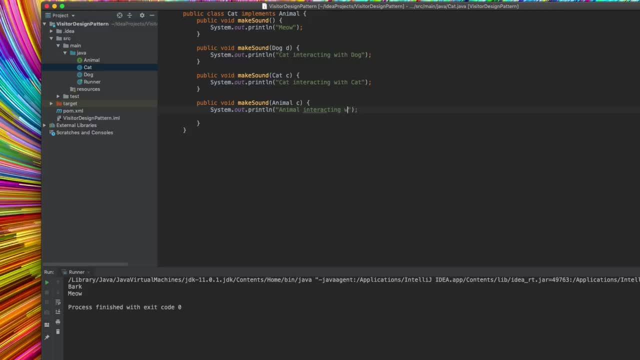 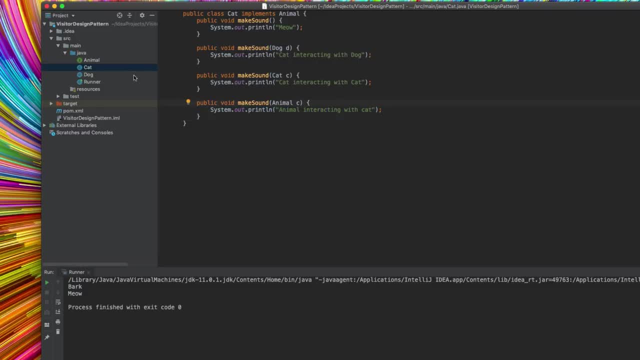 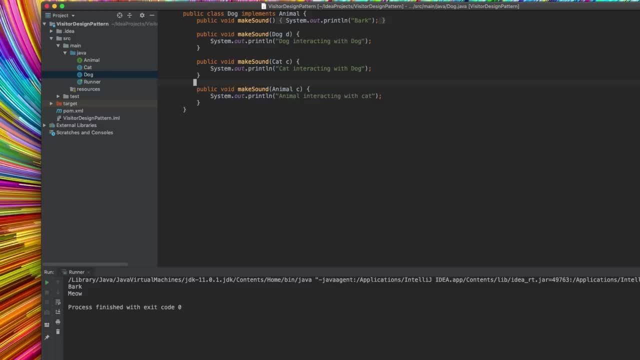 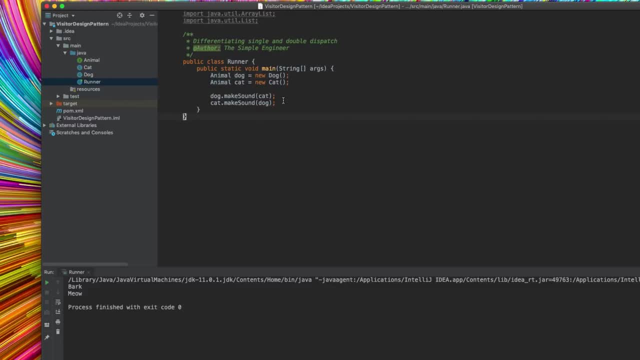 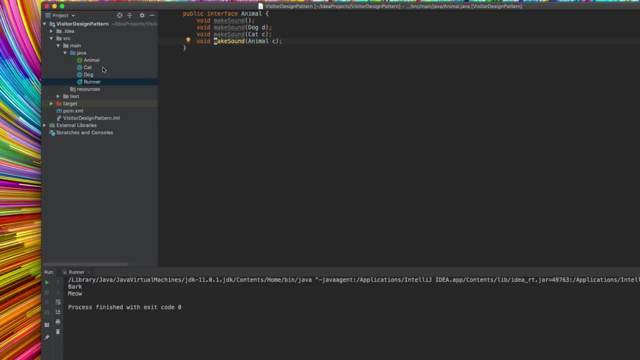 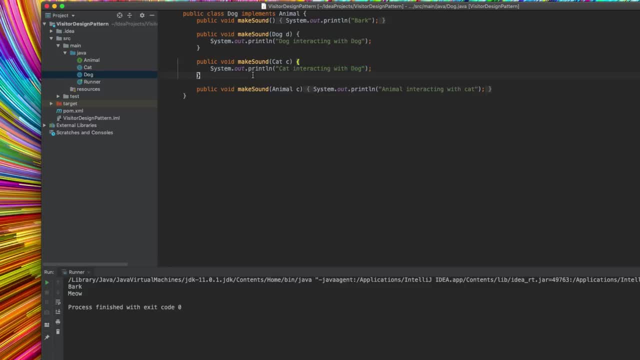 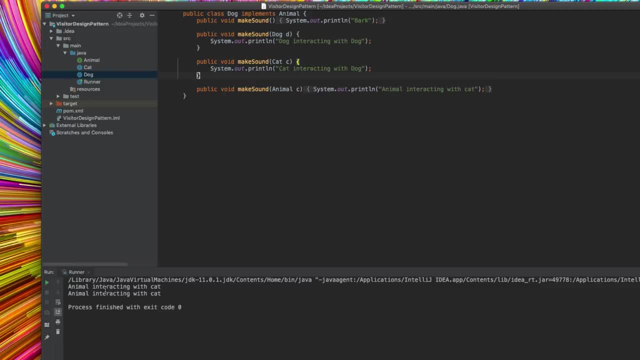 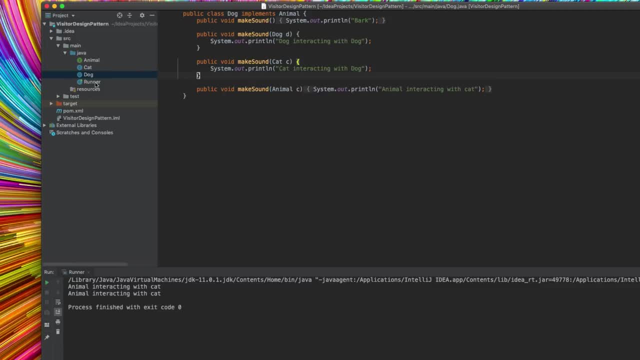 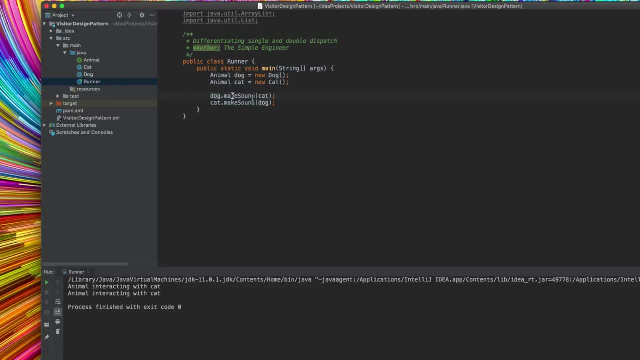 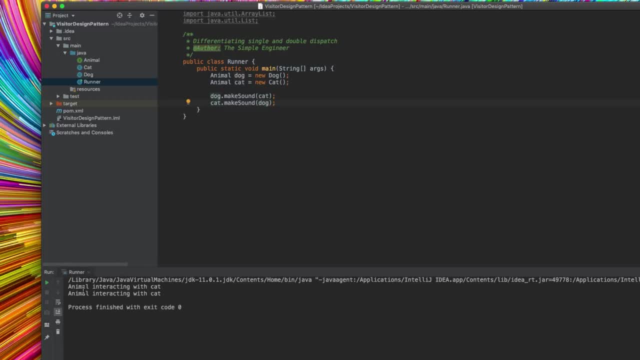 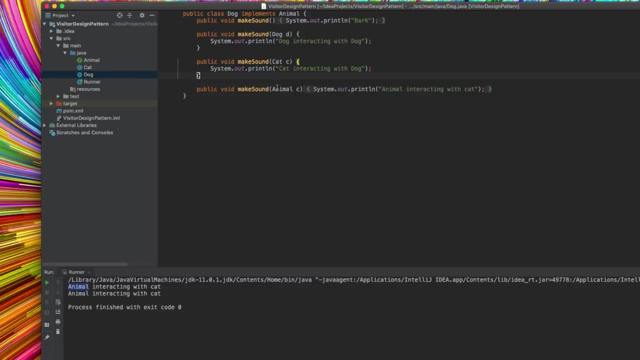 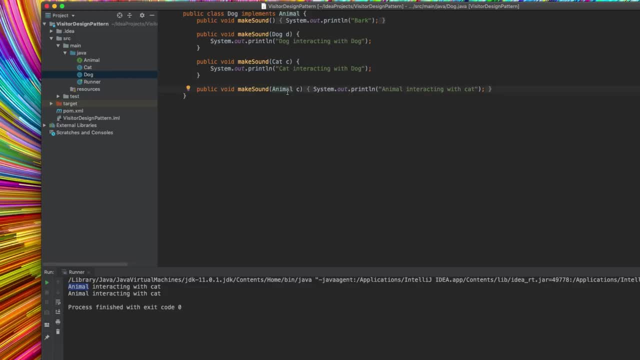 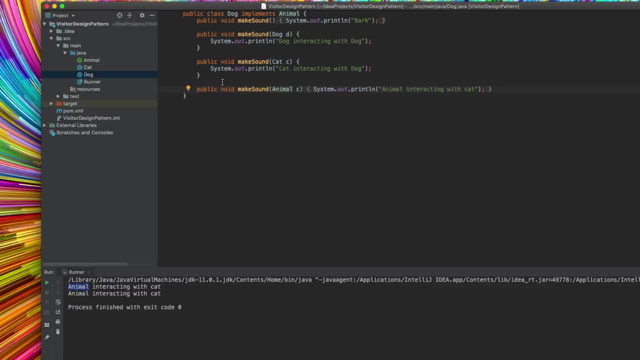 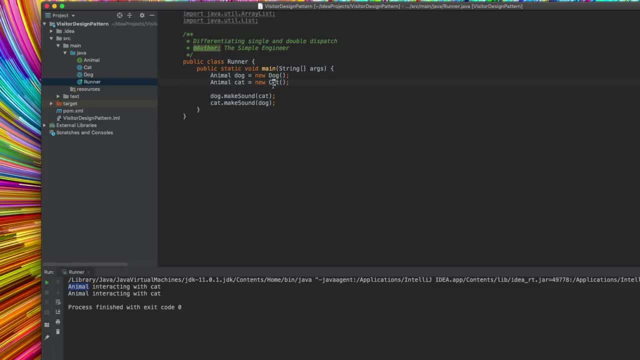 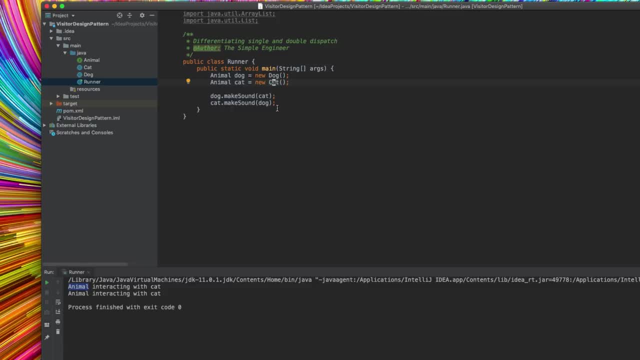 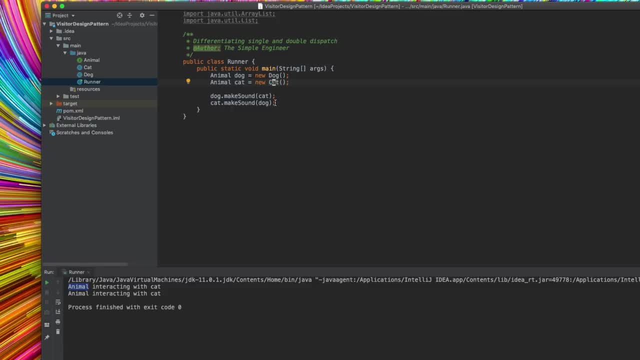 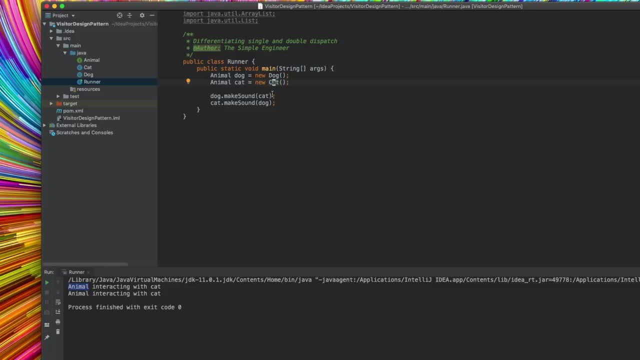 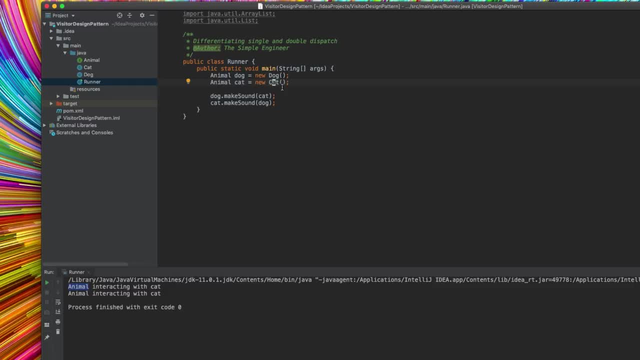 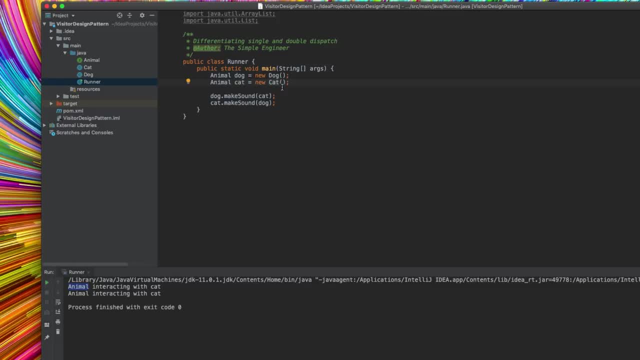 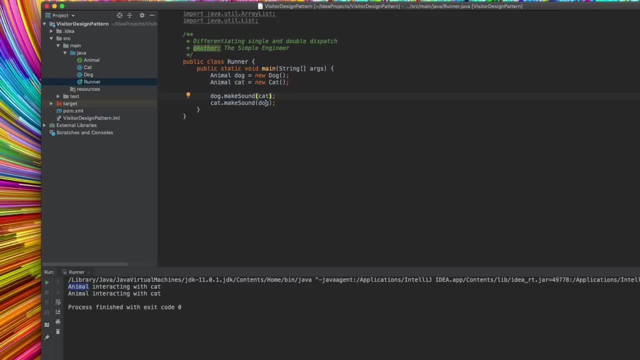 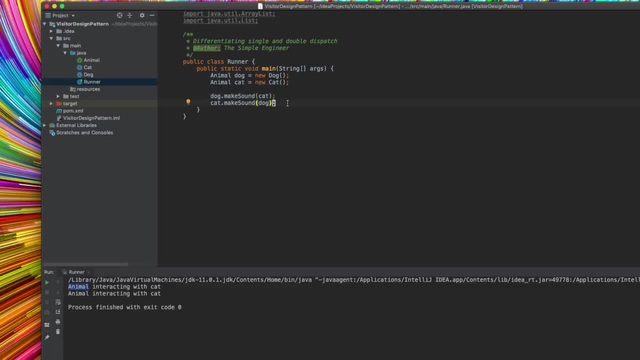 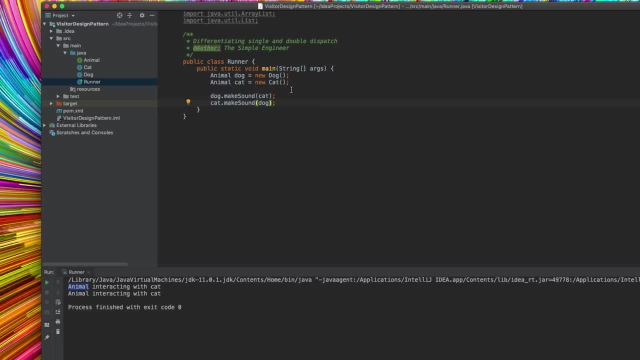 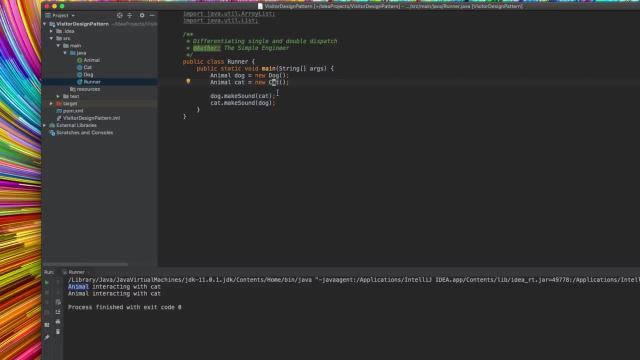 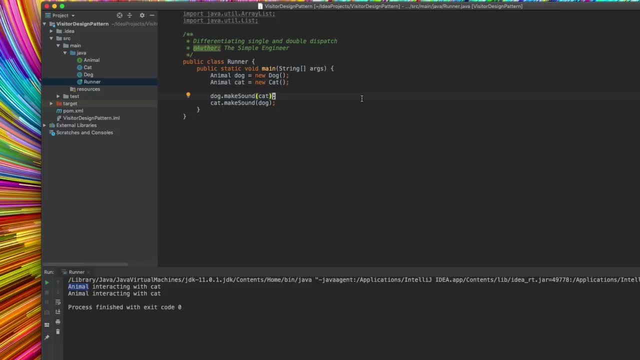 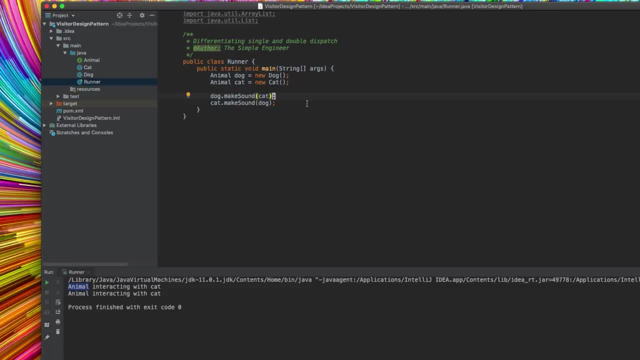 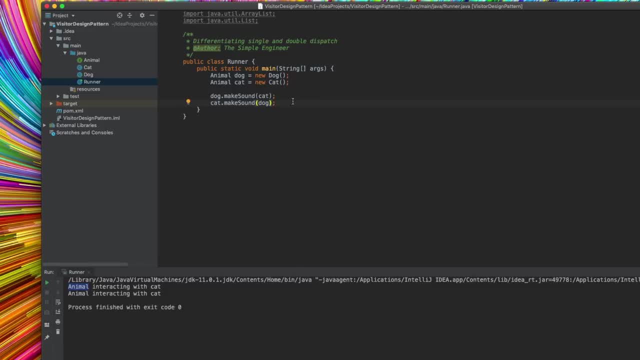 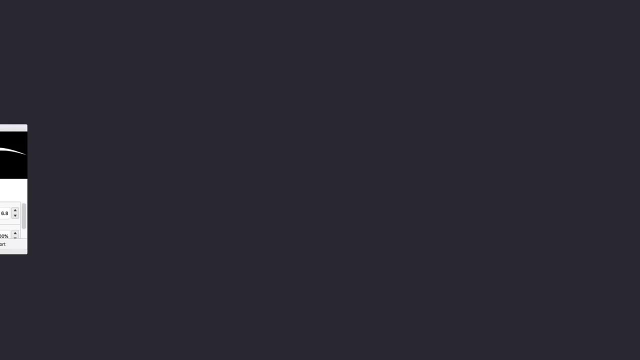 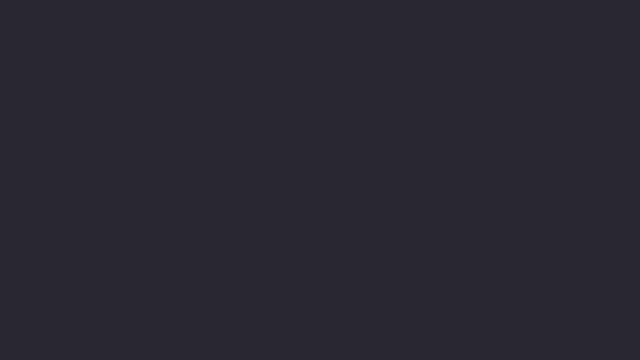 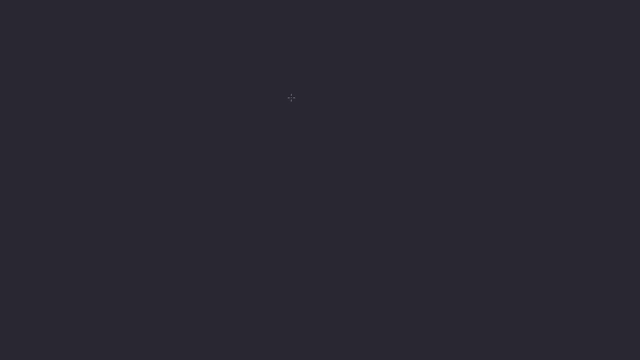 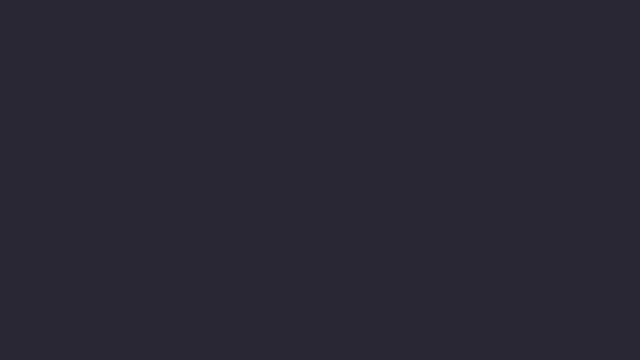 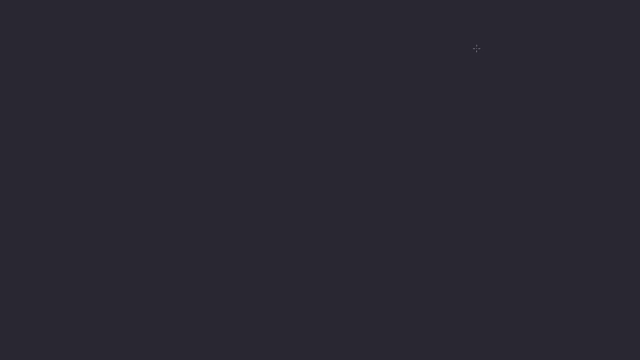 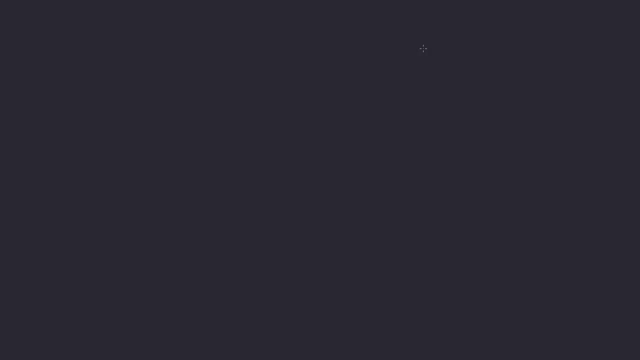 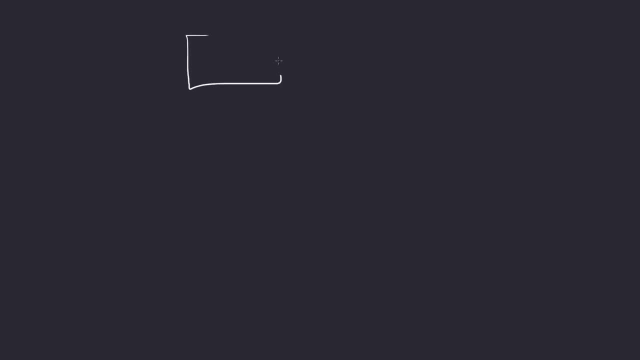 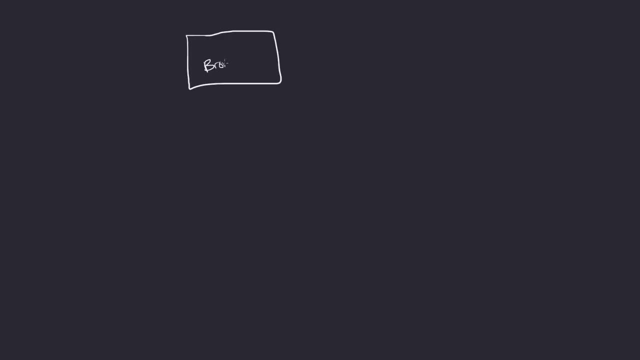 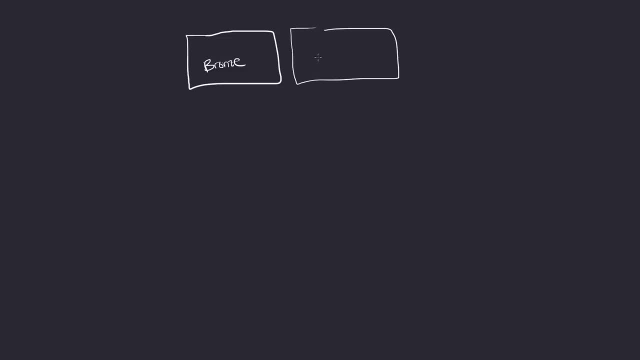 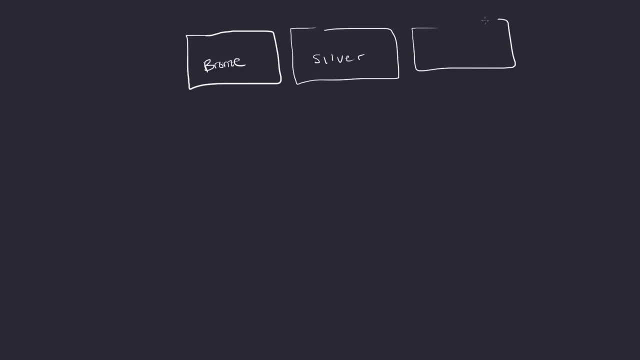 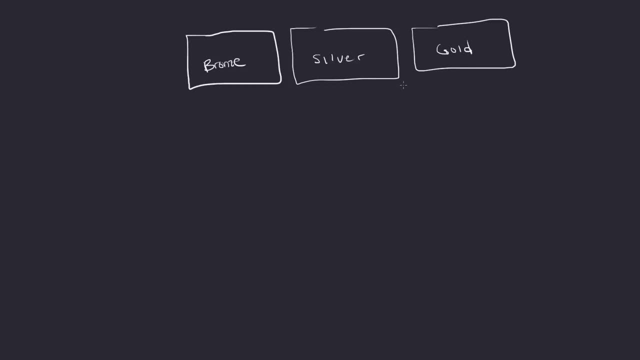 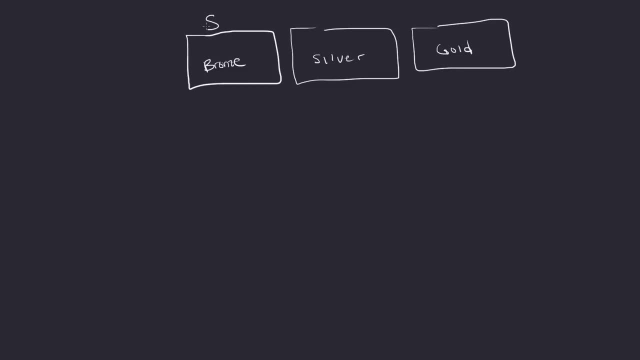 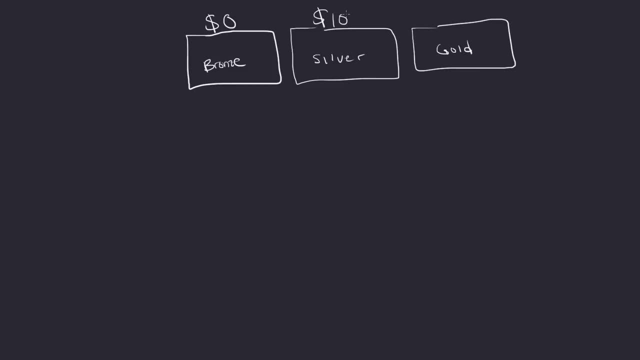 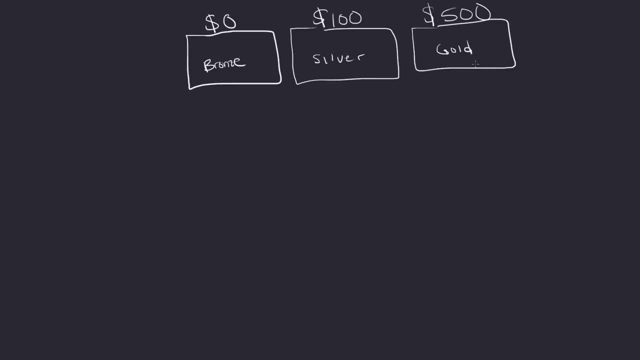 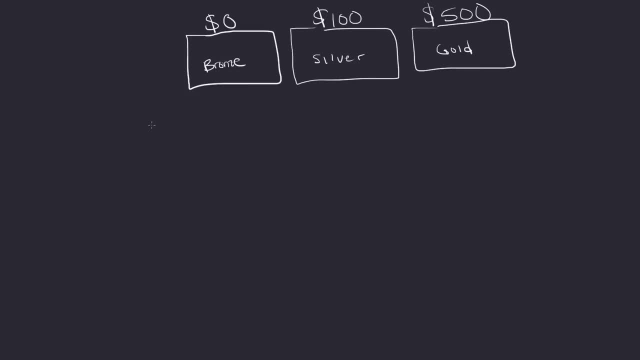 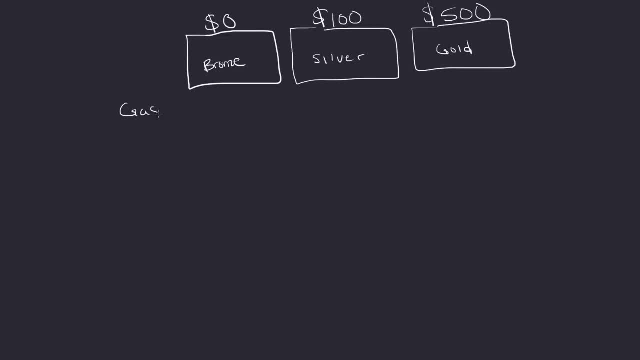 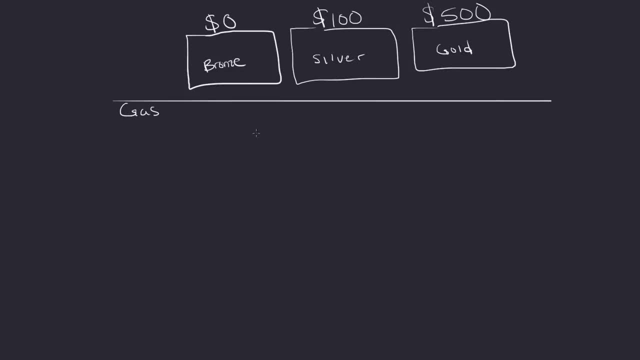 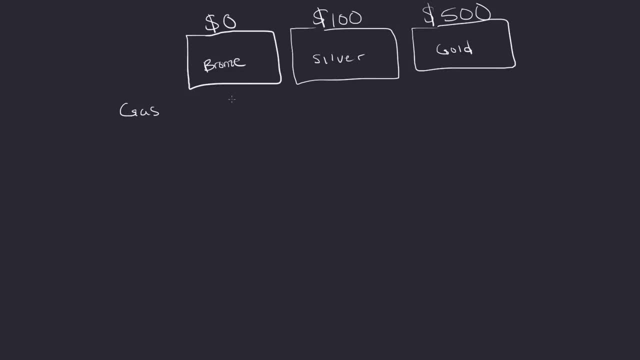 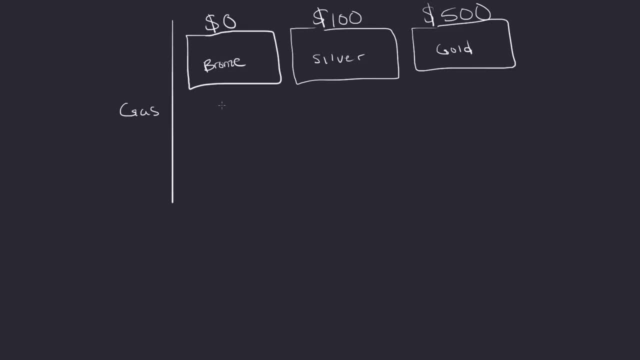 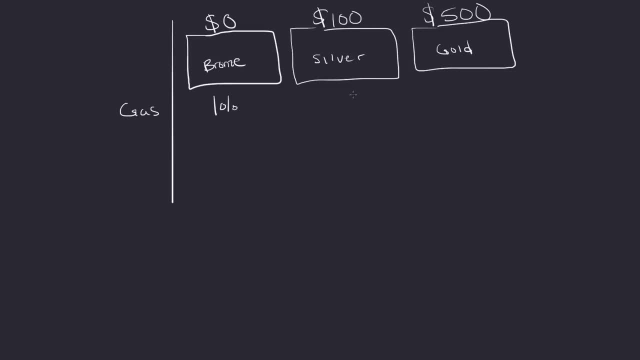 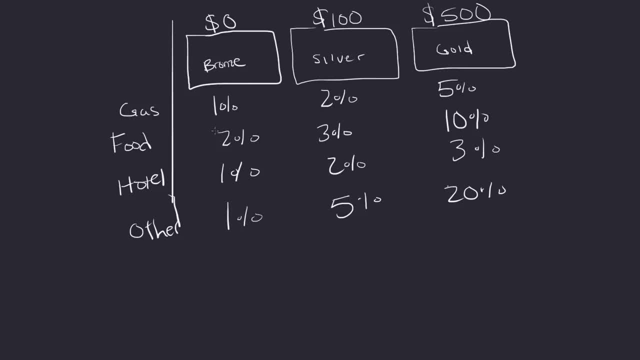 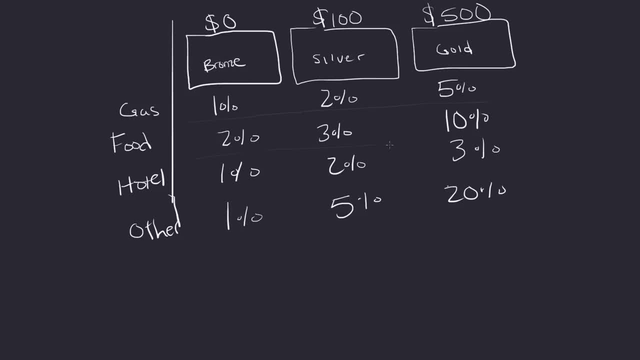 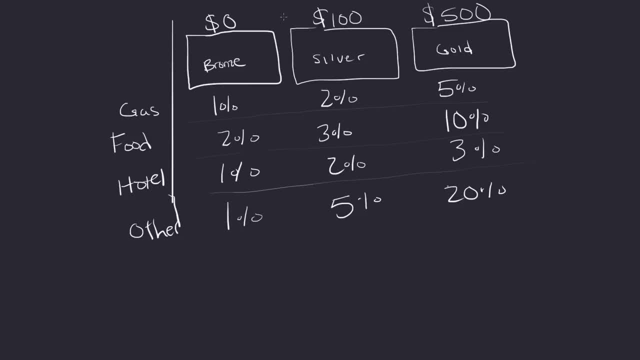 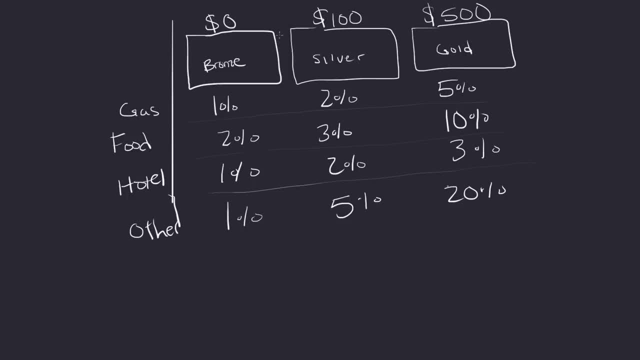 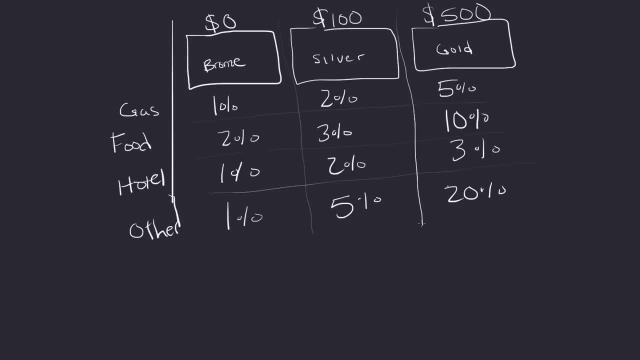 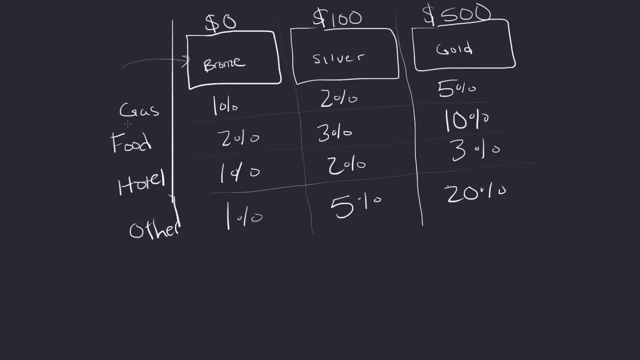 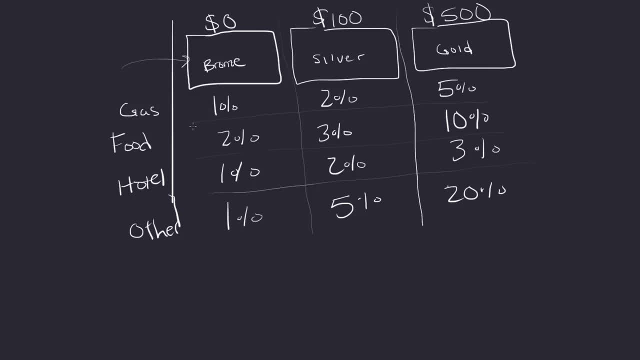 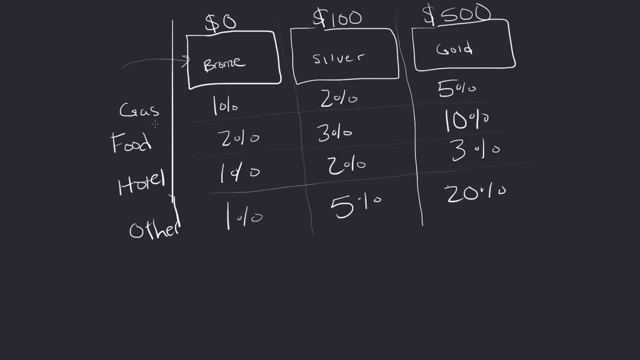 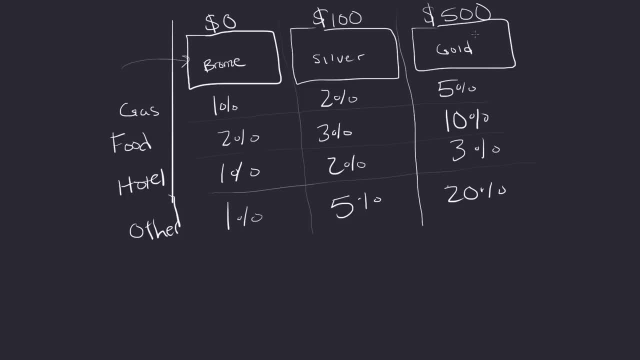 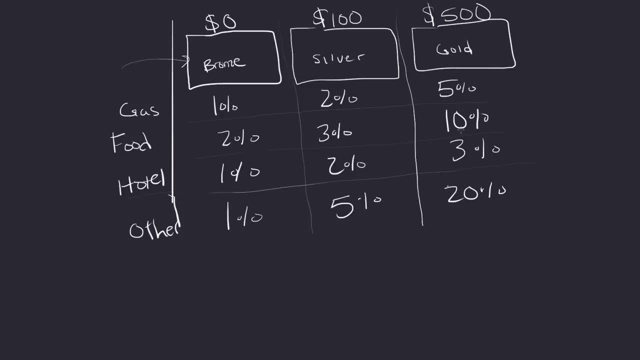 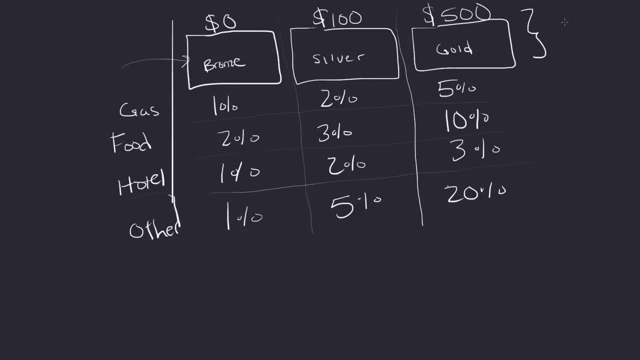 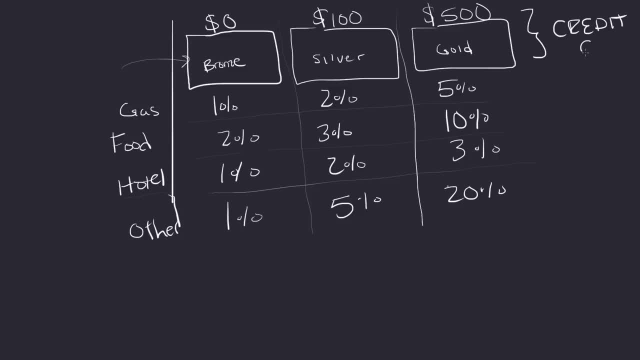 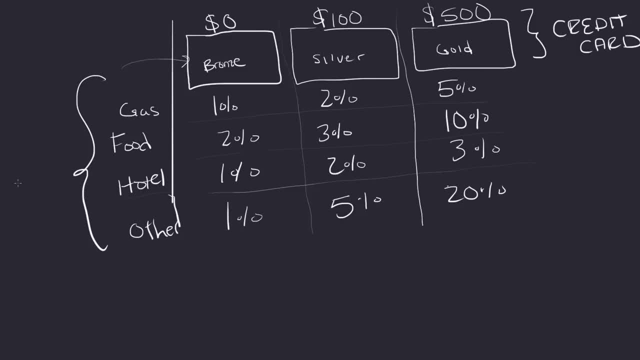 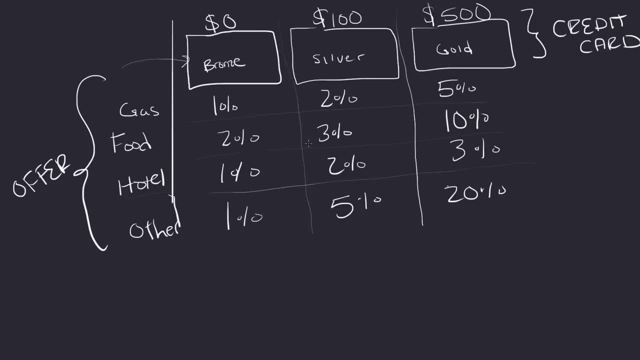 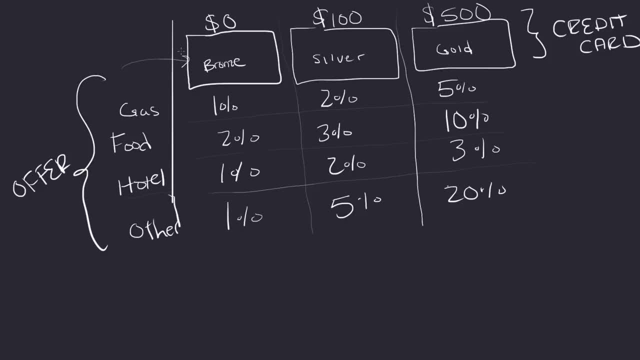 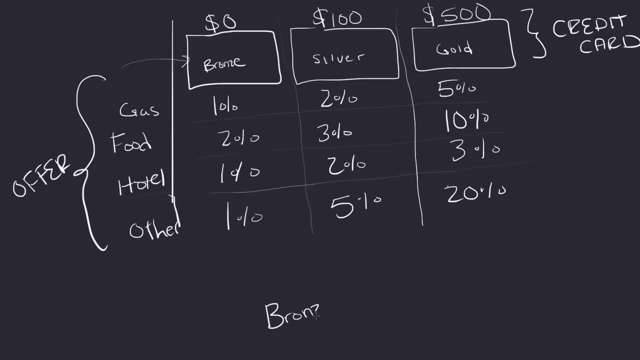 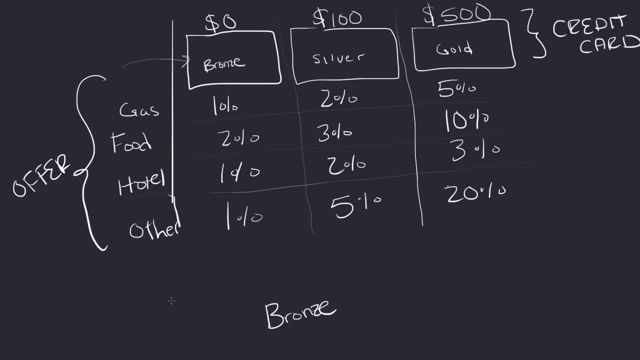 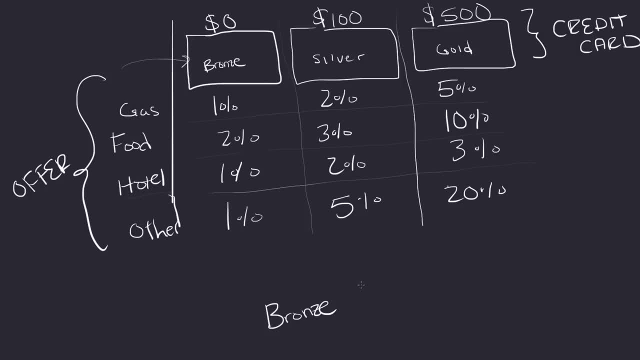 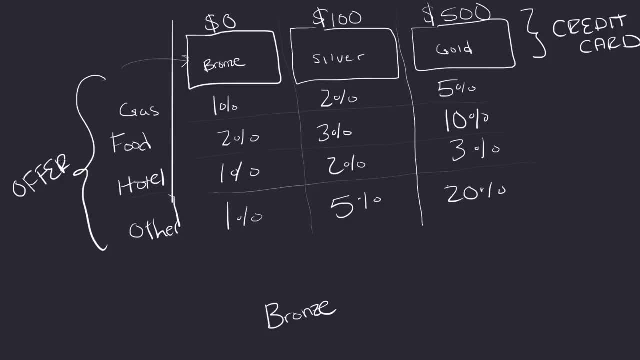 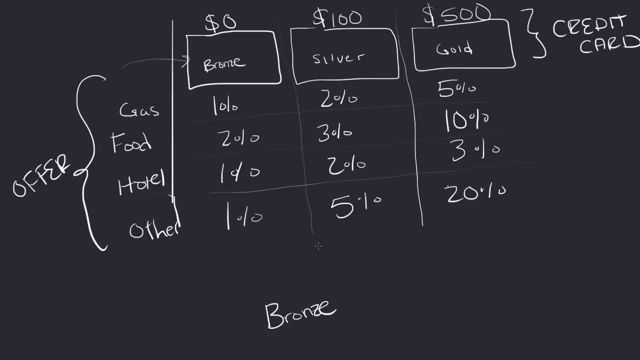 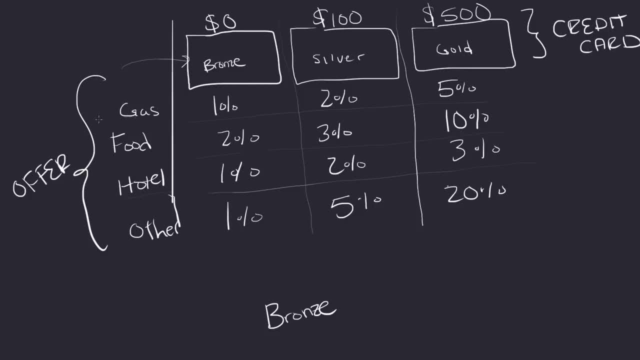 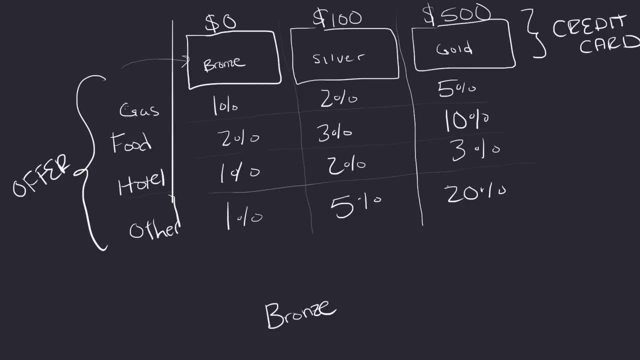 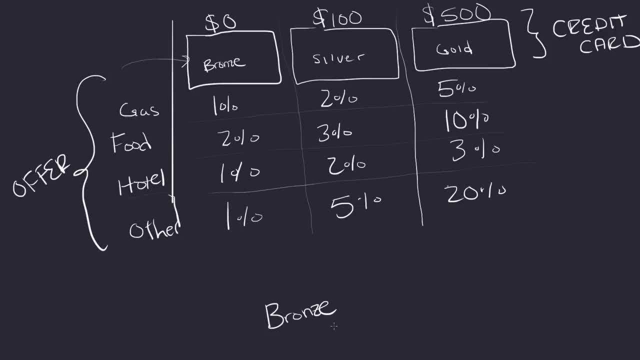 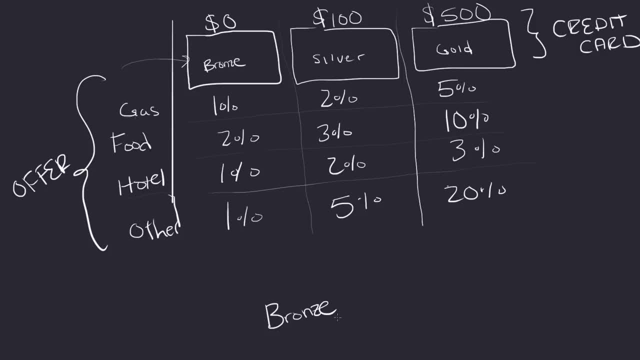 declare or instantiate two different animal objects- dog and cat- And we can declare or instantiate two different animal objects- dog and cat- And we can unrelated things. the bronze credit card is here to give you metadata about the credit card itself, not to tell you about other offers. that's what the offer classes are for, so we want to avoid. 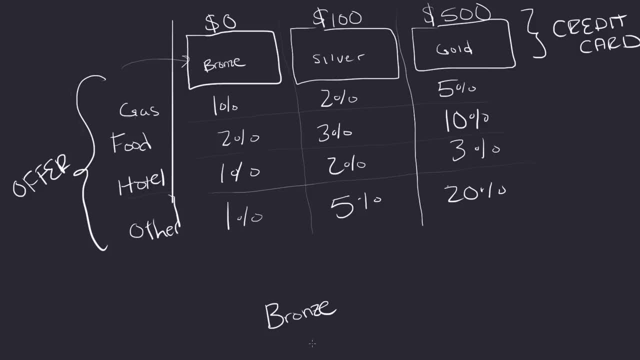 tightly coupling these offer computations. you know we don't want to have a compute cash back function, compute cash for every single you know gas offer etc. and then just have a bunch of these methods, because these methods will grow and grow and grow, and as we modify the original, 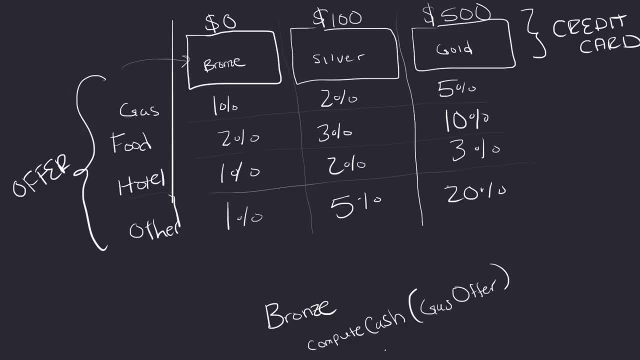 credit card interface. we're going to be breaking all of the concrete implementations. so the visitor design pattern basically says: how can we have just a generic concrete implementation for bronze, silver and gold and dynamically add these offers to the class? so that's what we are going to do. 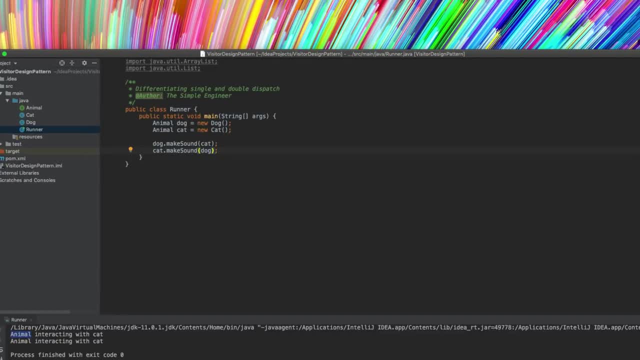 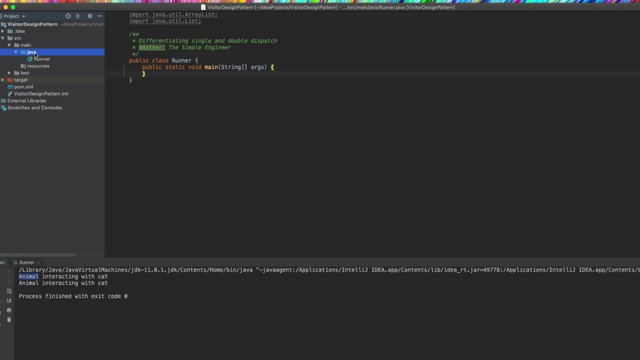 with the visitor design pattern. so we'll go: in intellij, we will actually just delete these methods, we don't care about them anymore- And in runner, we will just go ahead and delete this. So, like I said before, we are going to start with designing our visitor design pattern. 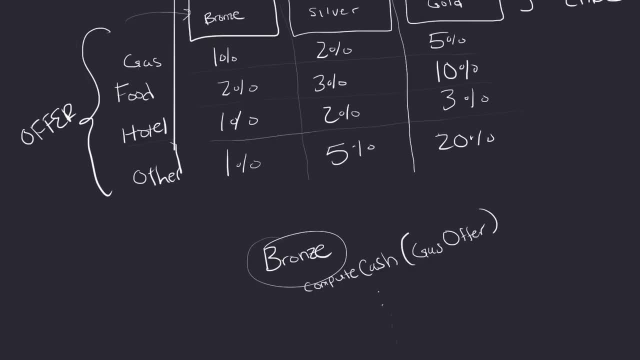 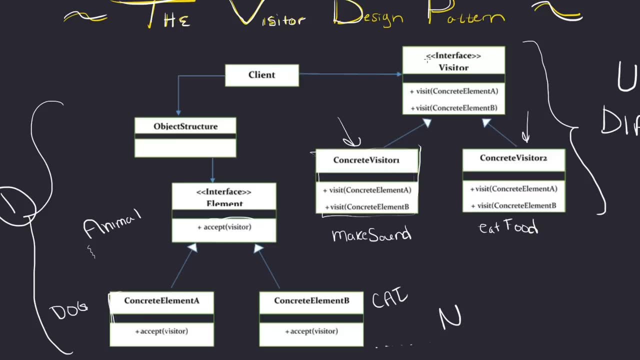 We already looked at this UML data structure before, so can just pull that up again. This is essentially the visitors or the dynamic operations that we want to add, And we've already discussed that we don't want to tightly couple the offers to the actual 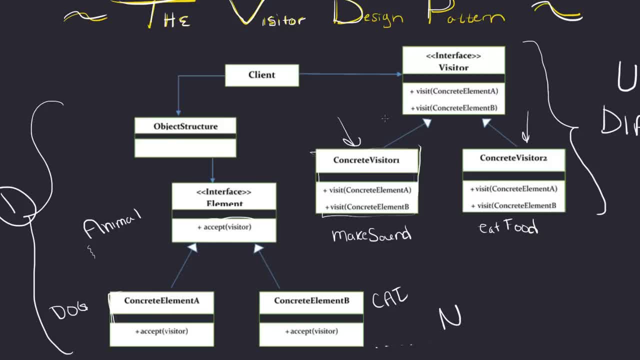 credit card types. right, That would be a bad thing. So what we're going to do is we're going to create visitors for the offer types. So this is going to be something like a gas offer. This could be a hotel offer. 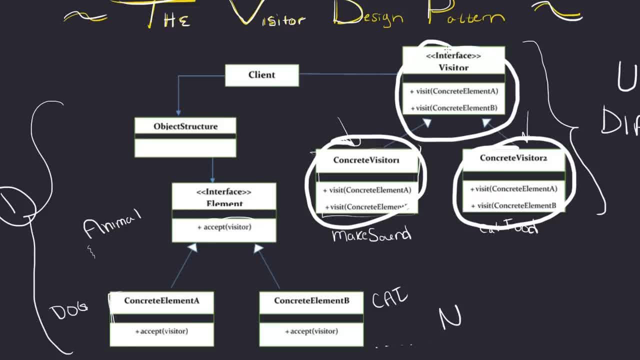 And then this is just going to be the generic visitor And this is just going to be for all of those different visitors. Likewise, on the first piece of the hierarchy, we are going to have a credit card interface and just implement bronze, silver and gold credit cards respectively. 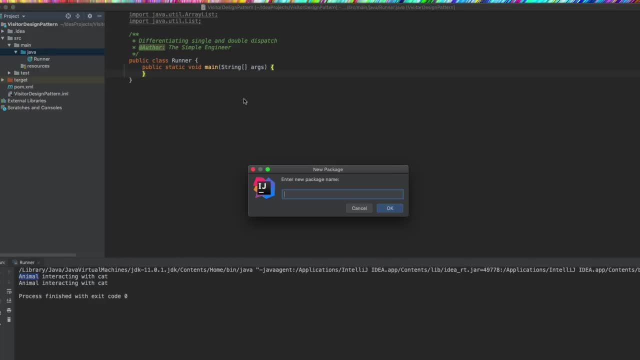 So I'll come in here and we can just segregate this in a cleaner way. So we'll just call this: create a package and call them offers. So, like I said before, we'll create a credit card interface. We'll just call this credit card. 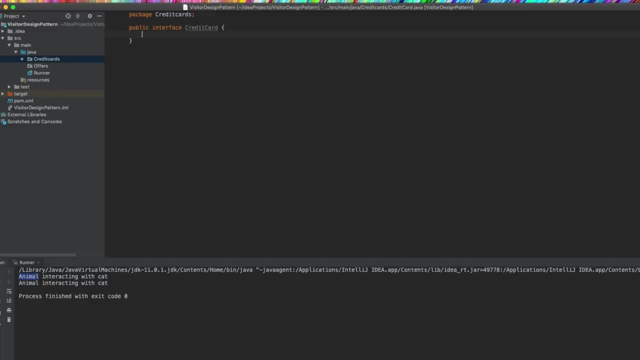 And, you know, maybe in the credit card interface we'll have something like get name and this maybe returns a string And we will have a new method in here called accept, And accept is going to accept a visitor, object v, which we haven't actually created yet. 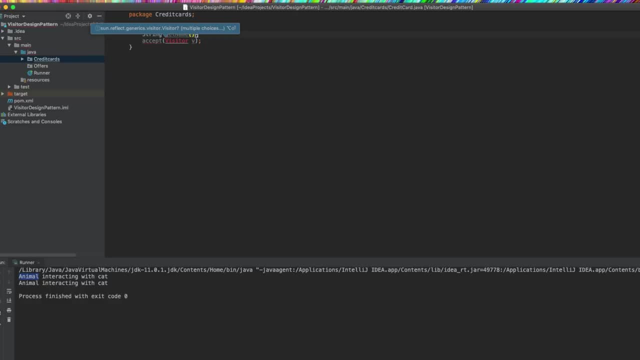 So we'll create that in a second. But this is going to be the interface for a credit card, So when I come in here, we'll go ahead and create a few credit card objects. We'll have a bronze silver. Okay, so we have a couple of errors here. 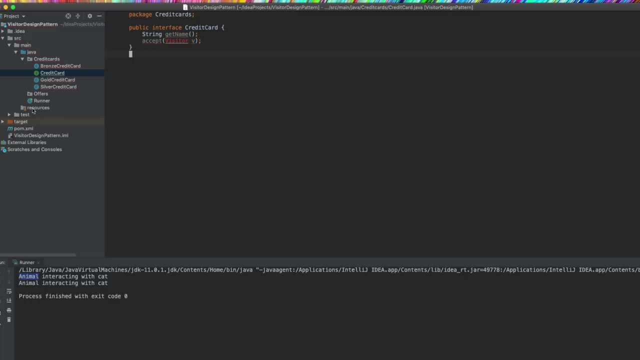 That's because we haven't created our visitor hierarchy, So let's go ahead and do that as well. We're going to create a new class here and it's just going to be actually an interface, and we will call it just the offer Visitor. 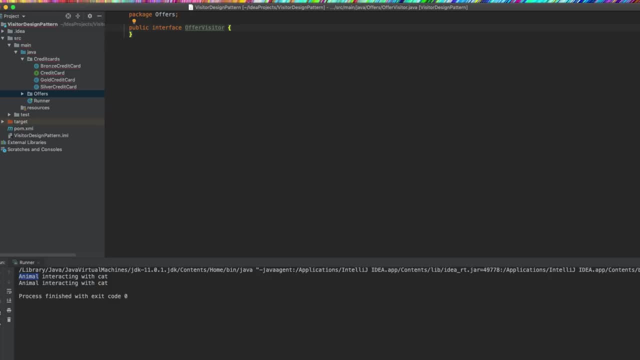 And the offer visitor is going to be the most generic form of offers that we add. that basically allow us to add new offers to credit cards without modifying anything related to the credit card itself. So I'm going to come in here and the different types of methods that we'll add is we'll add: 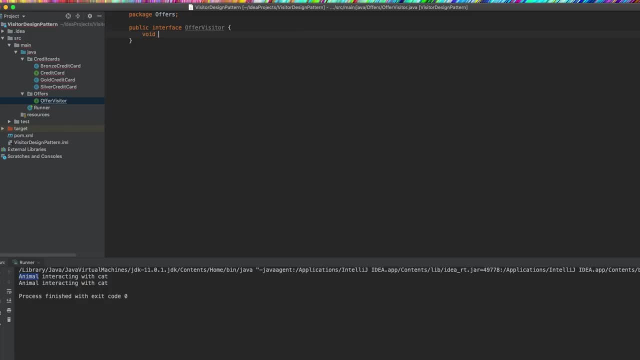 an avoid method called visit bronze credit card And it will take in a bronze credit card instance. We'll create a new method called visit silver credit card and it will take in a silver credit card instance And this is going to be the offer visitor. 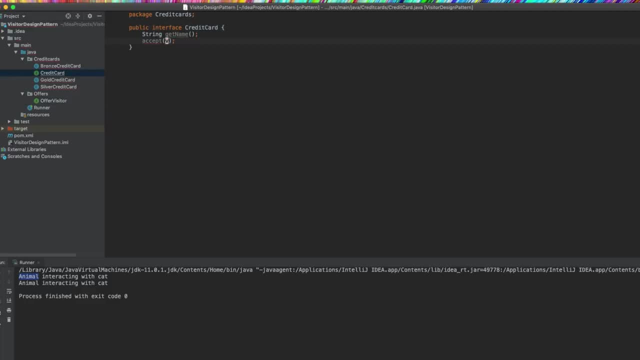 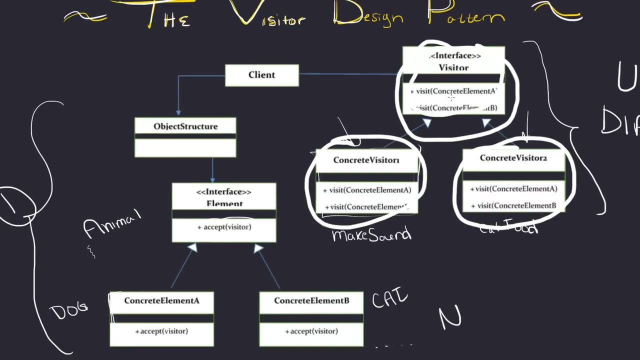 So now we can go into this original interface here and we'll just change this to offer visitor: Okay, And it will be avoid method Okay. So to kind of reference back at our UML diagram, this is the offer visitor that we've created. 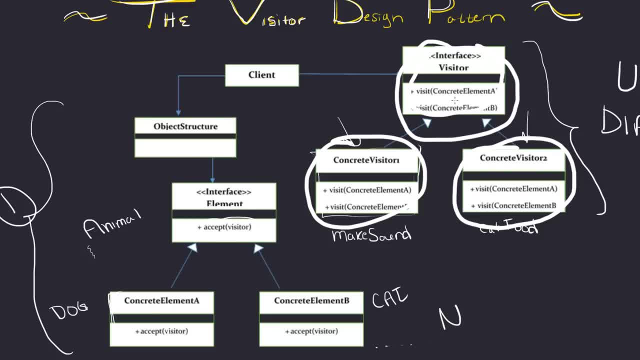 and it has a bunch of visit methods that are overloaded with the concrete types. And this is the credit card interface that we are designing right now, And you can see that it has the accept method and just one additional method related to credit cards, And now we're going to actually update the concrete credit card types to now account. 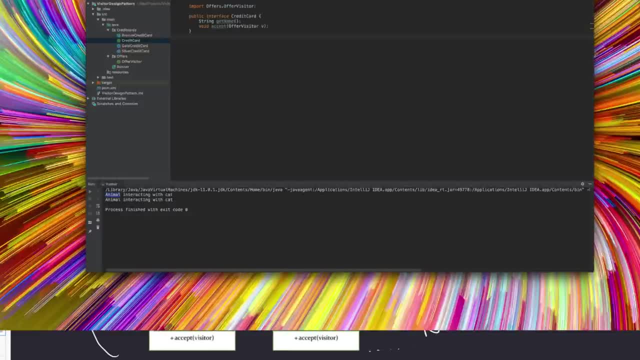 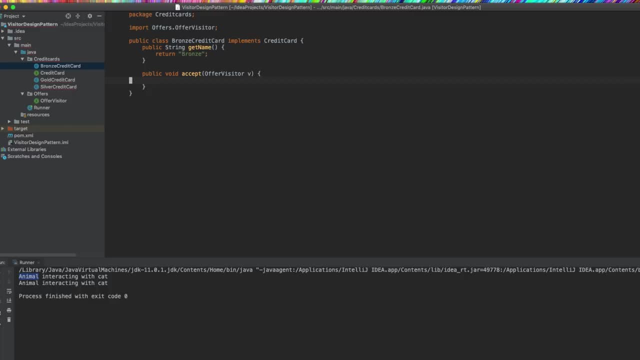 for this new method that we have added to its interface. So I'll go into bronze credit card. We're getting an error because we need to implement the accept method And all we're going to do here is we're going to call the visit bronze credit card method. 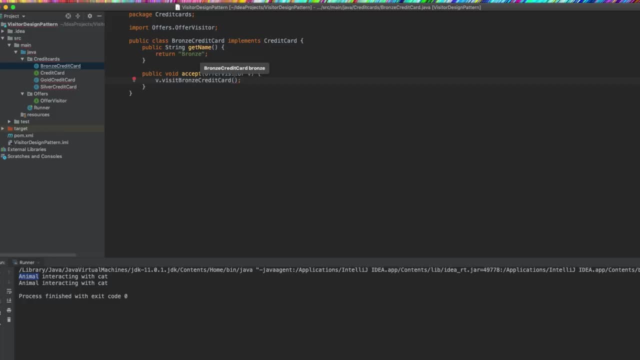 since we are indeed a bronze credit card And we'll just pass in an instance of our self. Okay, We'll go ahead and do the same thing for the gold credit card And we will call vvisit gold credit card and pass in an instance of our self. 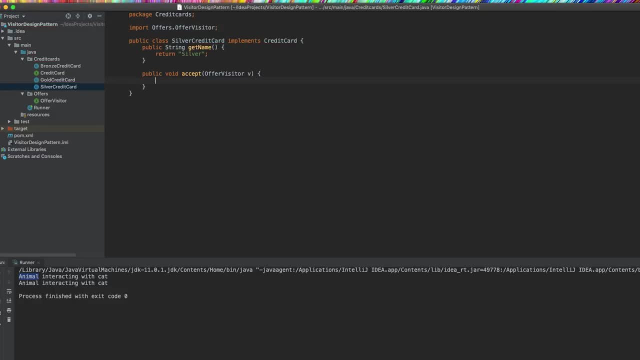 And finally, we'll implement the silver one, and it will be vvisit silver credit card with an instance of our self as well. So now we have no more errors, and what we're looking at here is this: accept method is essentially the entry point for extensibility, for extending any future operations dealing with offers. 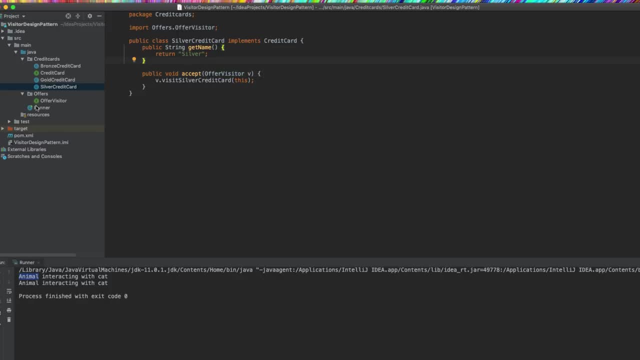 on this particular credit card. So if I come into the offer visitor, I have one offer visitor and now we want to start adding, you know, potentially cash back offers to figure out, based on the type of thing that we're purchasing, what is going to be the cash back value. 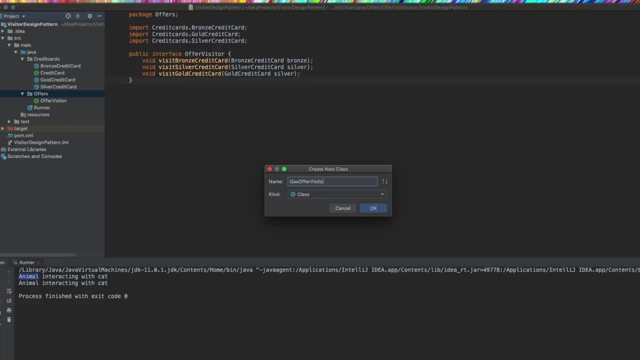 So I can come in here, Okay, And I can say gas offer visitor, and the gas offer visitor is going to be an offer visitor subtype and it's going to take in all the different types of credit cards. So once I go here I can say we are computing the cash back for a bronze card buying gas. 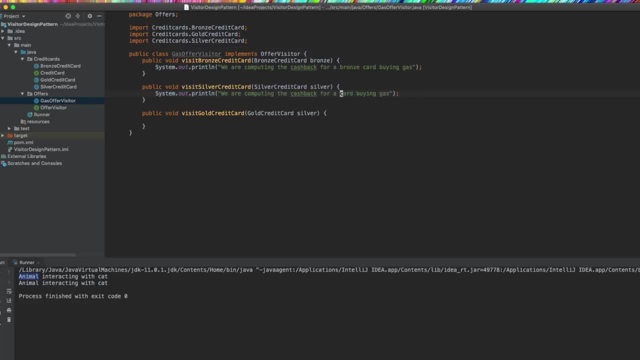 Now we can do the same thing For silver credit card, and we can do the same thing for a gold credit card, and that's just for gas. So we'll do one more to really drill down the idea and we'll call it a hotel offer. 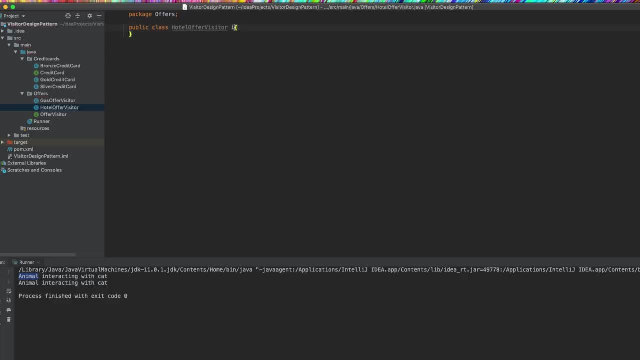 hotel offer visitor, And this is also going to be of type offer visitor, and we'll implement that and this is going to say almost the same Same thing. So we're computing the cash back for a bronze card buying hotel and this is going to be. 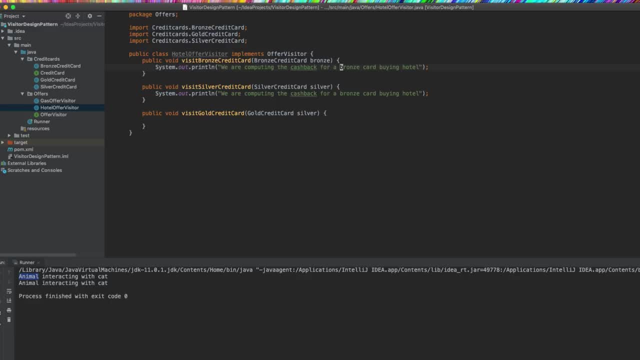 a, actually, this is going to be a bronze card, This is going to be a silver card buying a hotel and this is going to be a gold card buying a hotel. Okay, so now we're done, and what have we done exactly? Well, what we've done is now we're visiting. basically, we have these totally decoupled. 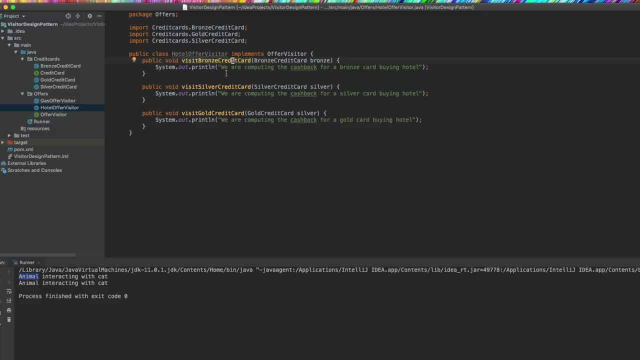 operations that we're still performing on each different type of credit card, but these operations don't clutter the actual credit card type. They only had one job and it was to return the name. We didn't want to have to clutter this with a bunch of different operations and there's 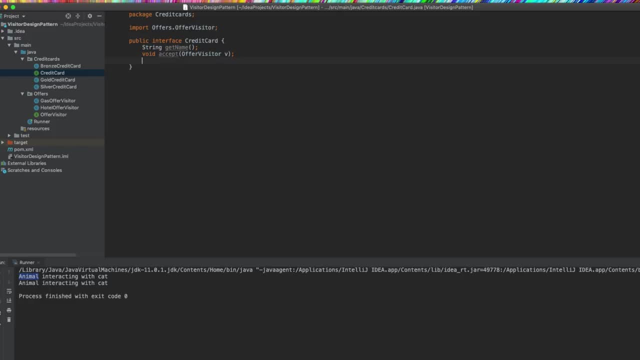 a lot of reason for that, Because if I were to come in here and I had to make a new method and it was called compute cash back for gas and then it took in a gas offer, for example, the issue that I would have to do is: now I just broke the underlying implementation of every single credit card. 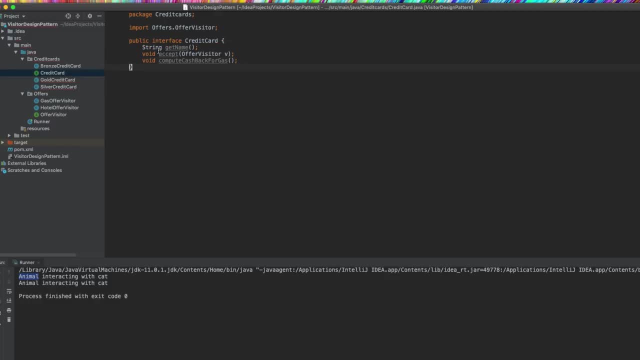 type You can see, I get a compiler error. So the second that we change the API, we break the implementations of all the subtypes, and that's something we want to avoid, Whereas now I've just added two new operations dealing with all of these credit card types. 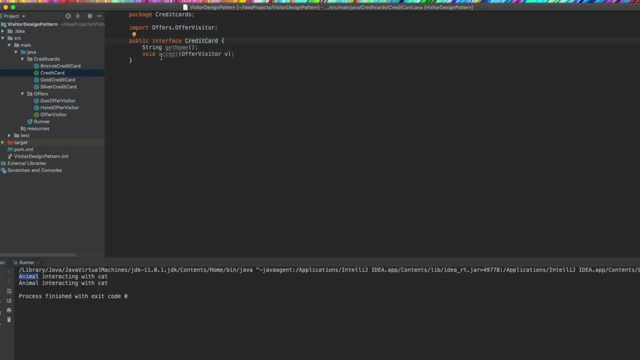 and they're totally decoupled and I didn't have to modify the original interface whatsoever. So how do we actually use this? What is this use case going to be? Well, what we do is we now instantiate one of the visitors that we're interested in. 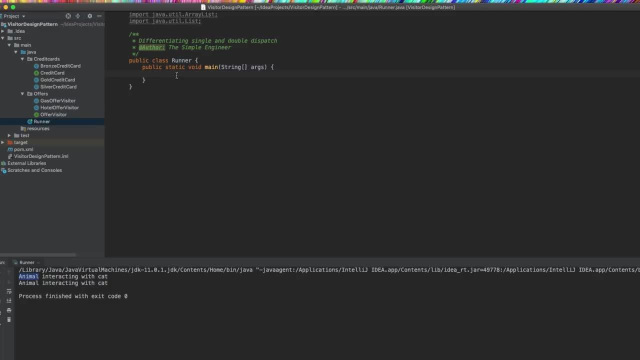 So let's say that we wanted to figure out the cash back that we get When passing in a hotel and a bronze card. what is the output of those two things interacting with one another? Well, the first thing that I do here is I instantiate a hotel offer visitor- new hotel. 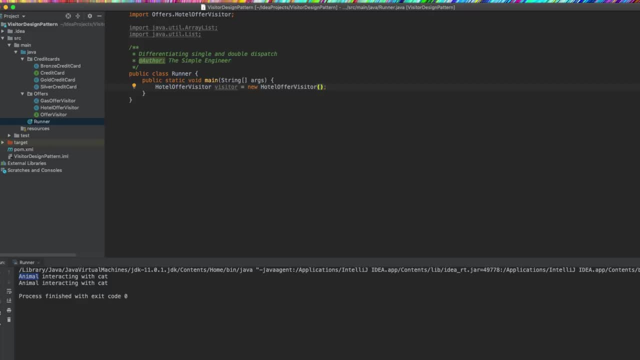 offer visitor. and then I come in and I create a bronze credit card. So let's say that in my pocket I know that I have a bronze credit card. So I come in here and I say: credit card bronze equals new bronze credit card. 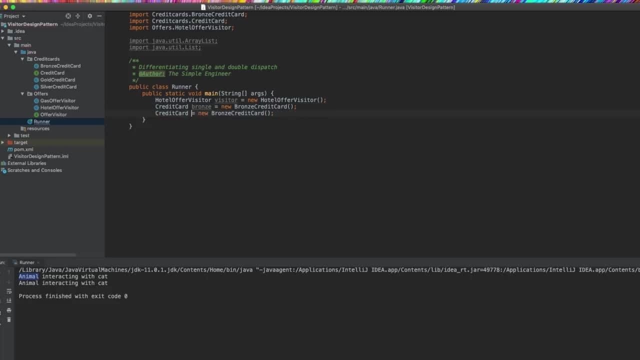 And I am going to- actually we'll just go ahead and create a few, So we'll create a silver one as well, And this will be a silver credit card, and we'll create a gold one, And we have our visitor. So, essentially, what's happening is we're trying to figure out the cash back of a bronze credit. 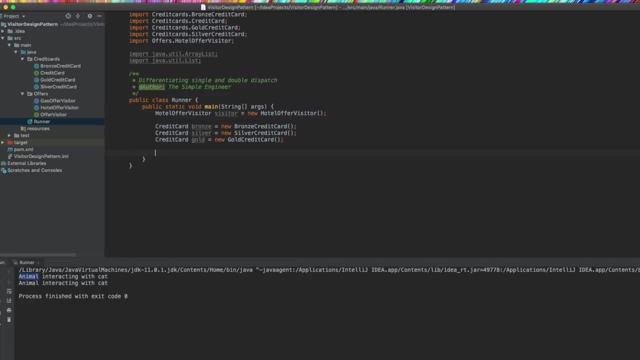 card And it is interacting with a hotel offer. So all we do now is we say, okay, well, bronze dot except, and it can accept any type of offer visitor. And in this case, what we're doing is we're passing it in a hotel visitor. 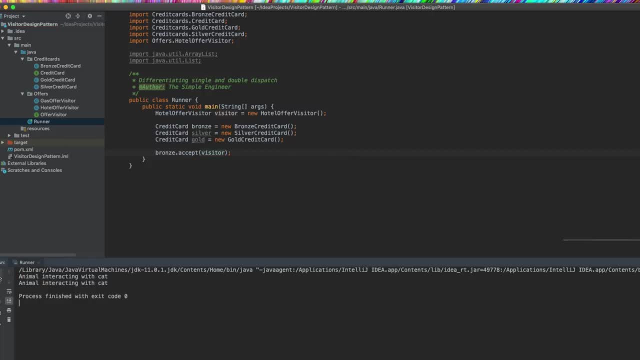 So when I pass this in- and now I run it- it should print that bronze is interacting with a hotel offer. And now we can see we are computing the cash back for a bronze card Buying a hotel, a hotel, and we can even get more generic. like i said before, the issue was we couldn't polymorphically. 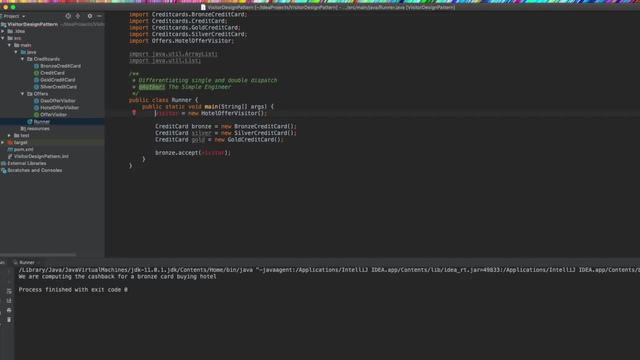 resolve two kind of abstract types right. so i can come in here and i can say: offer, visitor, pass that in. and if i run it again we should get the same result. so we are computing the cash back for a bronze card buying a hotel and we have two types that are basically being resolved at runtime. 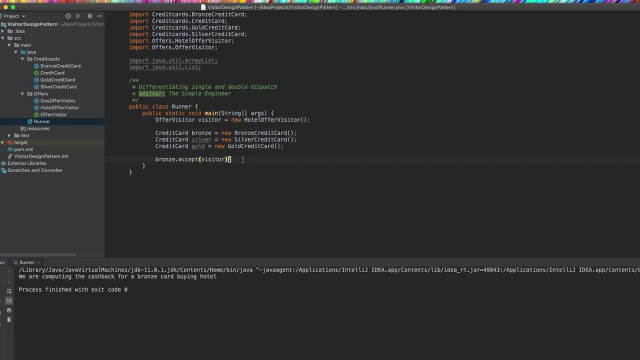 two polymorphic types that are resolved at runtime. so let's go ahead and do the same thing for the silver and gold cards, and we should basically be seeing that a silver card is interacting with a hotel offer, even though it's defined as an offer visitor, and we see bronze. 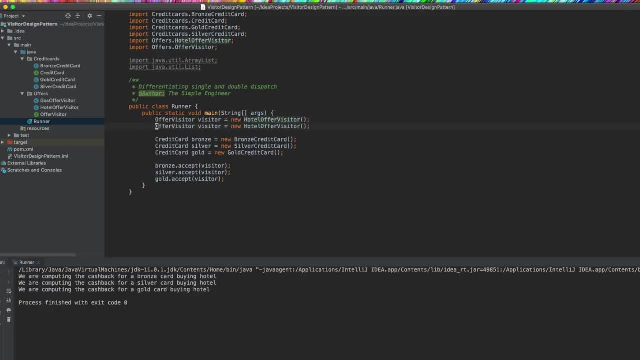 silver and gold respectively, and as we do this for different types of offers, you can see that the silver card is interacting with a hotel offer, and we see bronze silver and let's just call this visitor two. we can do this with a gas offer, and when we come in here and we 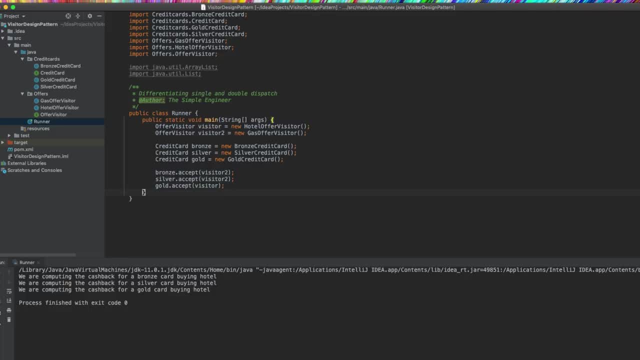 update this with visitor two. we should now be saying: we are computing the cash back for a you know whatever card. we're dealing with buying gas, so we'll click play. and now we can see this is the interaction of a credit card with a different type of offer. 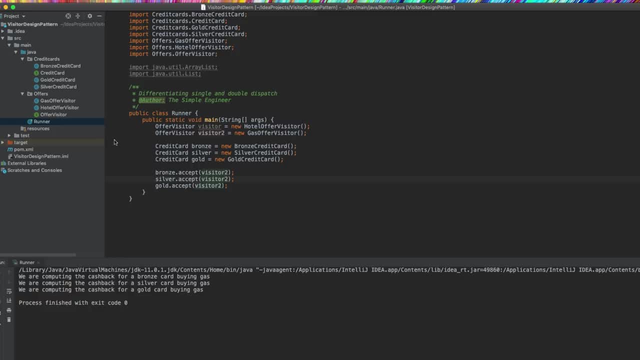 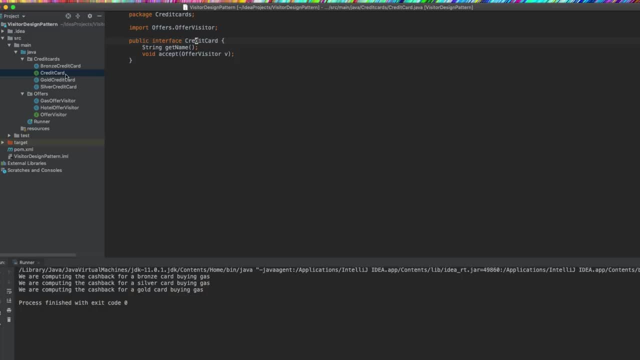 operations to the original data structure and original api. we've abstracted it in such a way that now we can have really really extensible operations or offers, in this case totally decoupled from the actual credit card concrete implementations. so i can add new operations as: 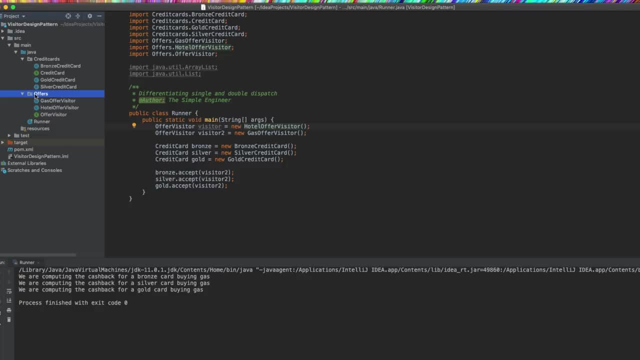 i please we could come in here and we could add, you know, uh, a restaurant offer, a food offer, grocery store offer- and compute cash back based on all the different credit card types dynamically and they can polymorphically resolve between two different polymorphic types- offer, visitors and credit cards- and this allows for really really fluid, extensibility. 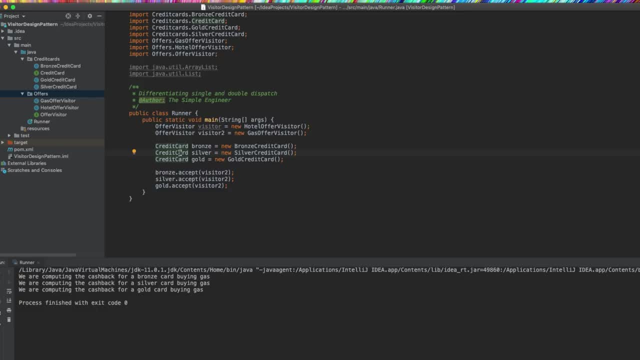 between our data structures. so the final question you may be asking: when do i want to use this design pattern? and you know there is no one all be all design pattern for every problem. but typically you want to use this pattern when your class structure is somewhat unchangeable. you don't change it often. however, the 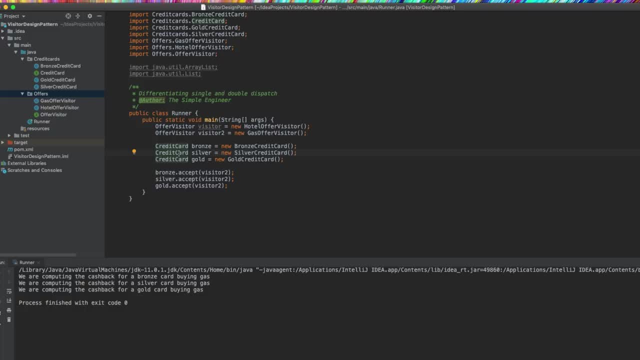 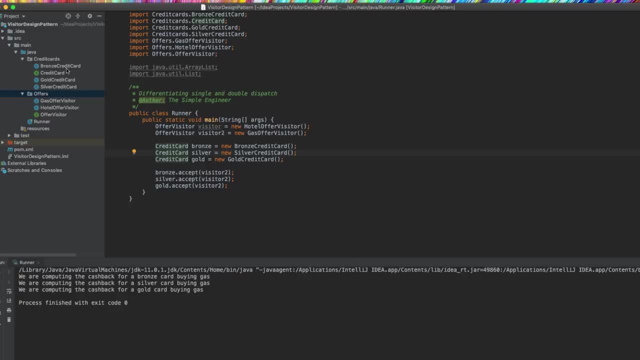 you know, like i said, restaurants, grocery stores, buying things at electronic stores- they could add all different types of incentives very, very often, but the underlying data structure of each credit card may not change as much as the different types of incentives, so that's a really good use case for 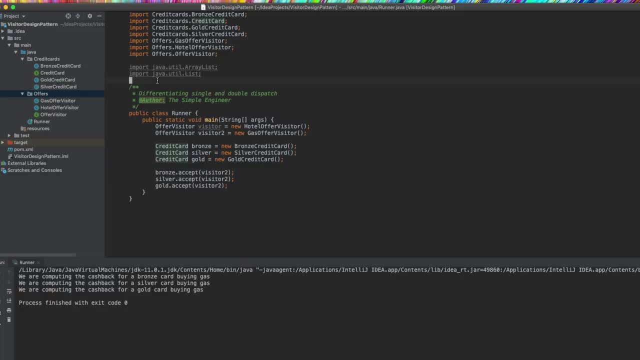 using something like the visitor design pattern, because i can come in here and i can create a new uber offer visitor and i can give cash back reward points for people using uber, and i didn't buy any of these credit cards at all to be able to do that. so that's just one use case in actuality,